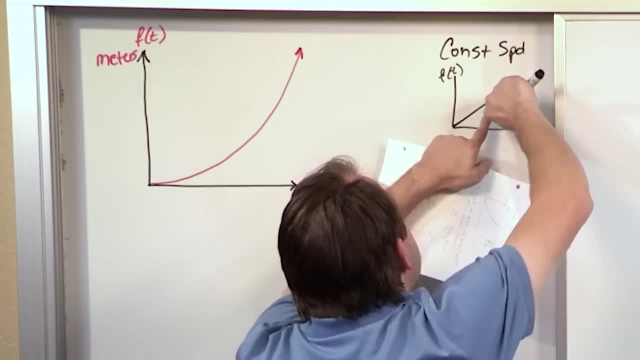 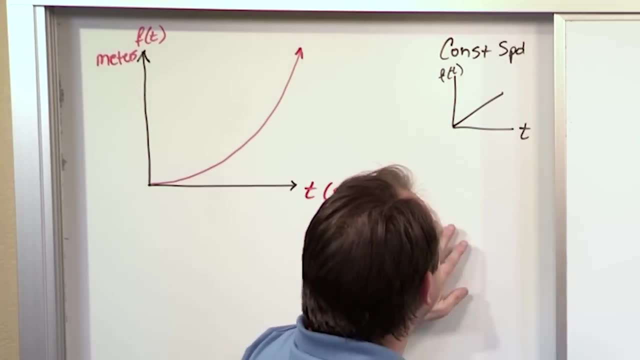 increments of one second. the thing has moved the same distance in the direction of travel, because it's a constant speed. So it's not a constant speed, It's a constant speed, It's a constant speed. So everywhere you move, the thing has gone up a same amount, Whereas here, as you go towards the 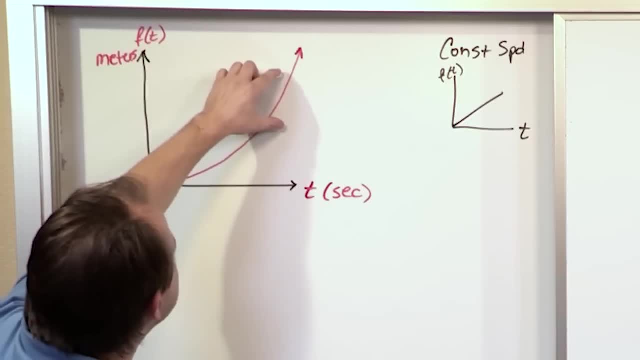 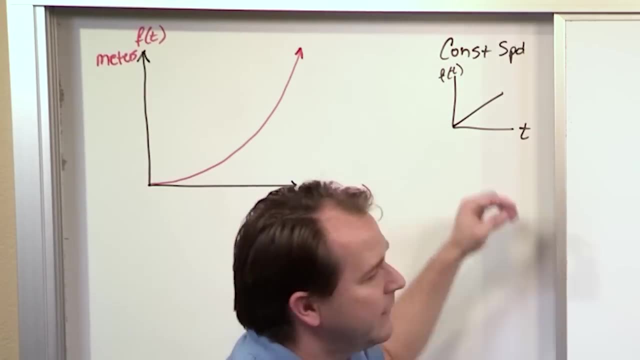 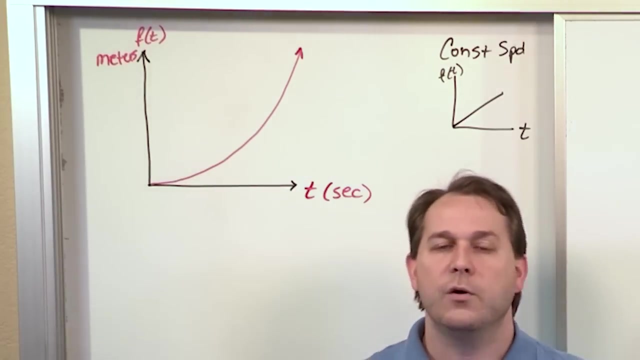 end of its travel, it's going up as far as its altitude, much, much more than it is when it first starts. So the question is: when you're in fourth grade you look at problems like this: A car is going 30 miles an hour. Let's calculate whatever. Or the car is going two miles in one minute. What's? 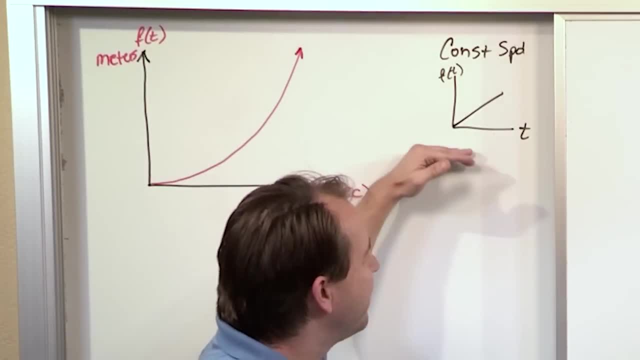 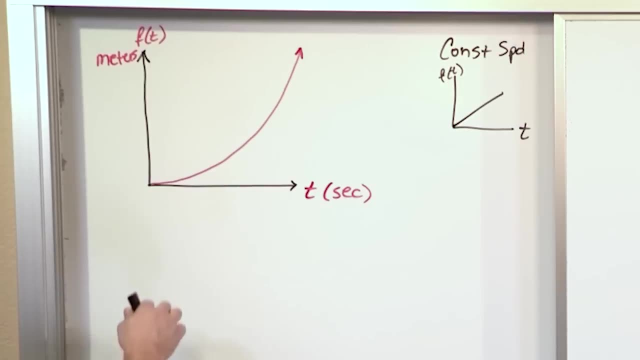 its speed, Assuming it has a constant speed. So we were doing problems like this. But in calculus you start to do more complicated problems. So how do you define the speed of this rocket? Well, we've already determined that the thing is going faster over here and it's going slower here. And 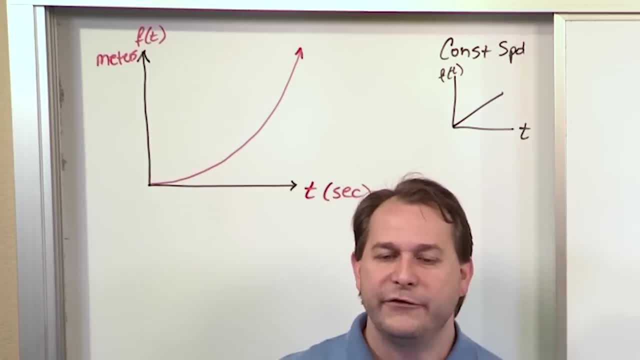 in fact, if you've ever watched a rocket launch, you know that that's true. As soon as the booster lights, it's barely moving right. But then, if you keep on watching it through a telescope, you can see that it starts cooking when it gets off the launch pad, because it's accelerating. 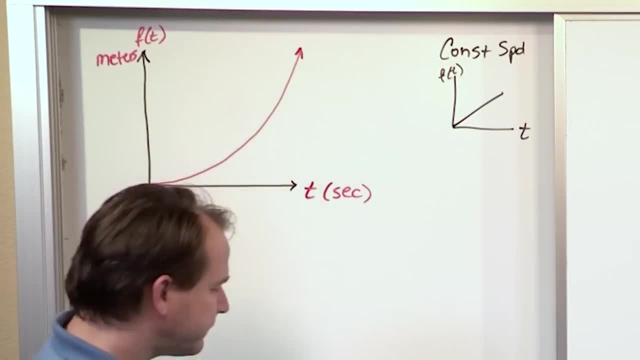 It's moving faster and faster and faster and faster like this. But, as we said before when I started, a good place to start to study the velocity here because, for instance, we know the velocity is pretty small here and we know the velocity is pretty high here, but we want to be. 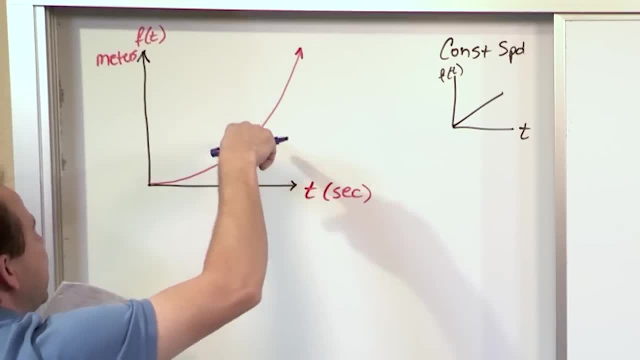 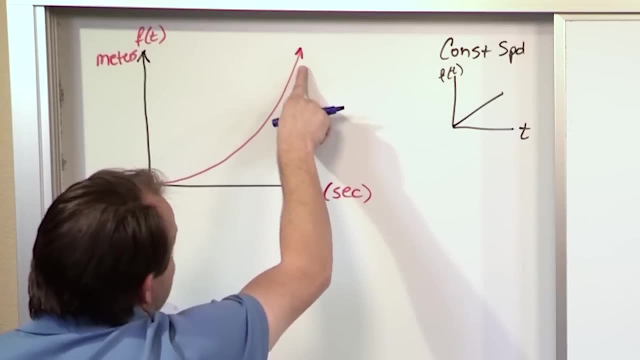 able to calculate, not the average velocity. We want to be able to calculate the velocity at this point in time, right here. How fast is it going? Or we might want to calculate the velocity right here, at this point in time: How fast is it going? This should be a higher velocity than this. 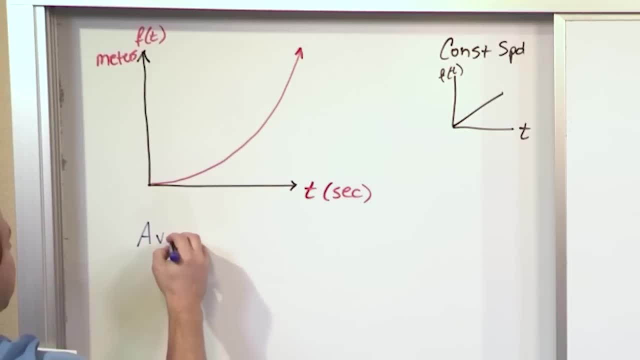 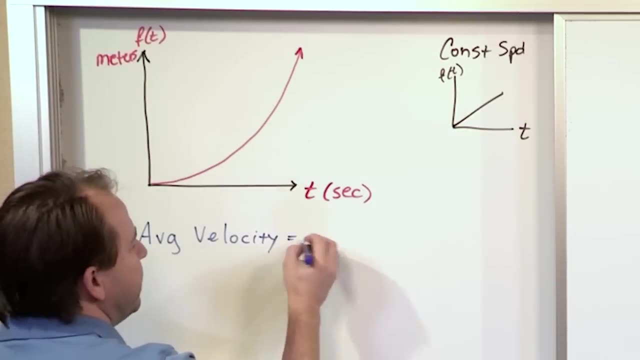 but how do we do it? Well, let's start with the concept of the average velocity. This is not going to be the answer, but it's the place to start. So we know that velocity, as we just talked about a minute ago, is distance, Distance traveled divided by the time it takes. 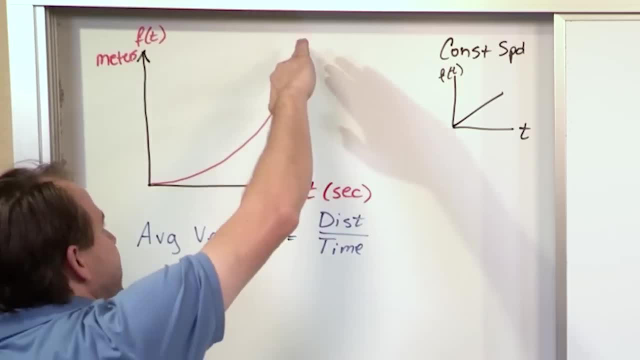 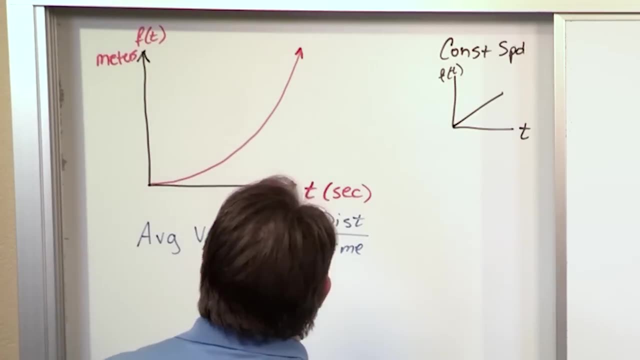 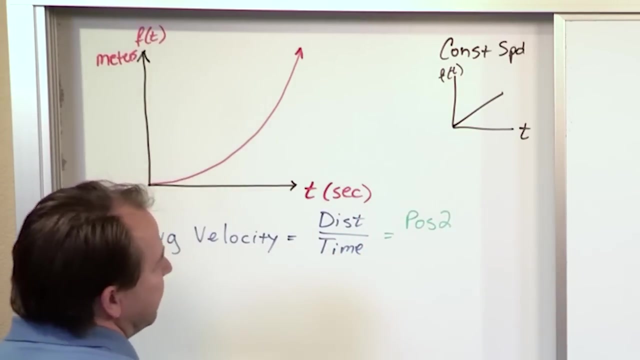 to go there. So if I wanted to get an estimate, a crude estimate, of the velocity at some point in time on this rocket path, then basically what I would do is I would figure out how far the rocket traveled, which would be the position two, the final destination position. 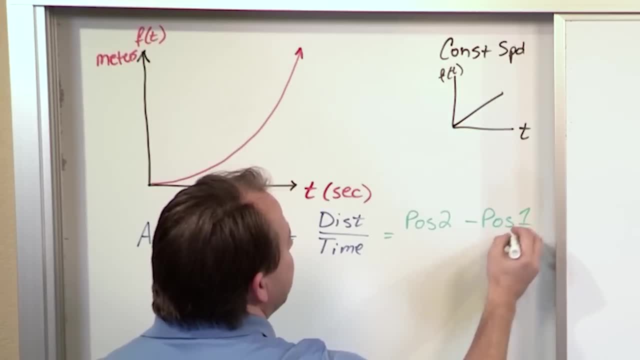 Minus the initial position wherever I'm starting to start my watch from, and then I'm counting how long it took for this thing to happen. So it's T2 minus T1.. So it's not really perfect because you have to look at two different points in time, and I already told you that I want to. 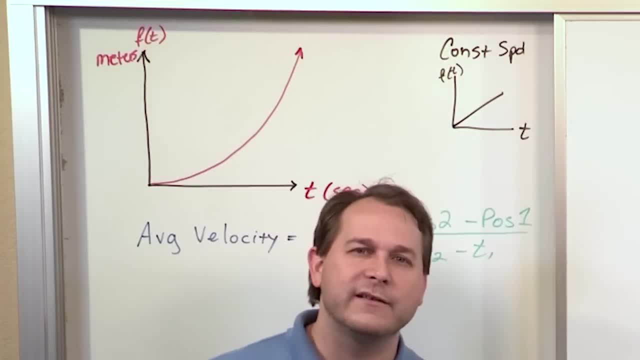 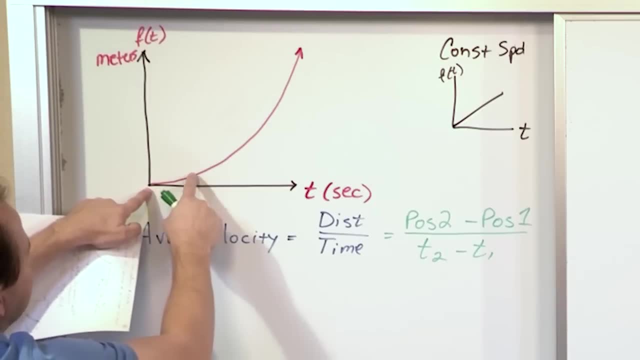 find the instantaneous velocity. But we're going to start here because it's a crude approximation. So, for instance, if we want to know roughly what the speed of the rocket is, here we'll start our watch here. We'll pick a few seconds in the future, maybe here And between these two. 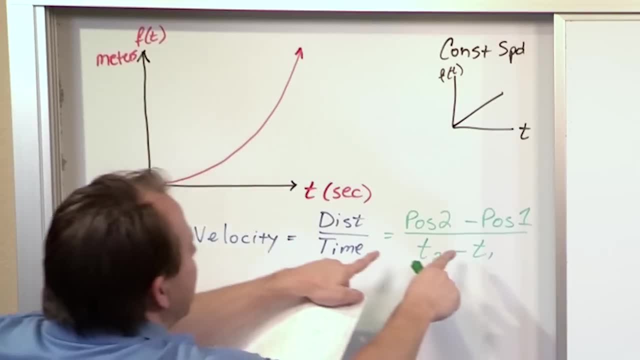 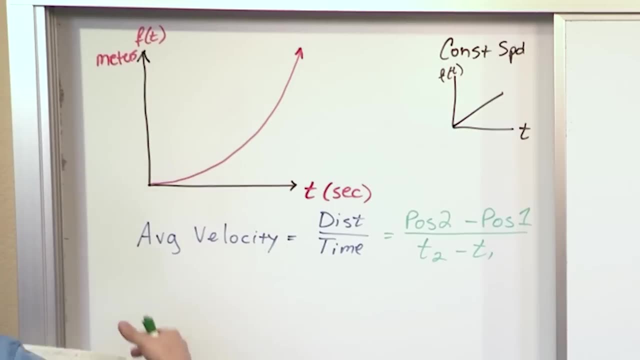 points. we'll figure out how far the thing traveled up and we'll figure out how far the thing, how long the thing took for it to happen. We'll divide these numbers and we'll come up with a crude estimate. We're calling it the average velocity. We know that the actual velocity 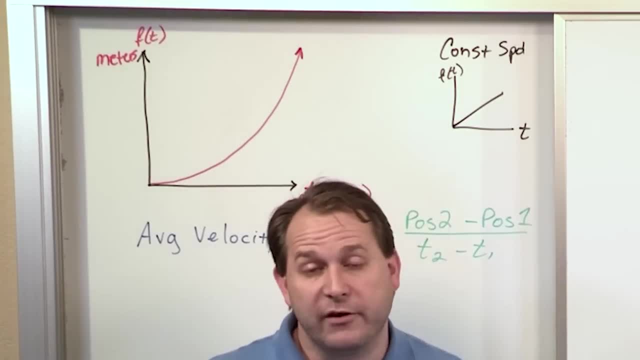 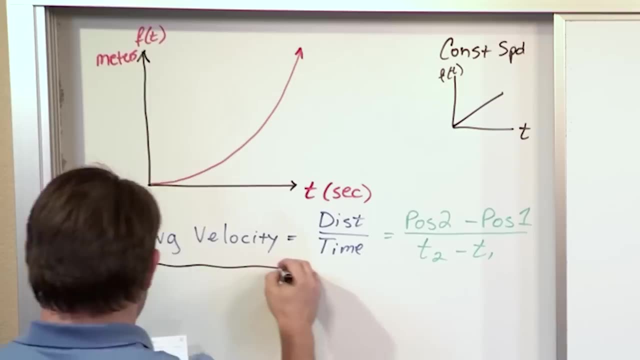 is changing in that window. but we have to start somewhere, so we start with the average velocity. So I've kind of gestured enough with this picture. I want to draw a little more. well, let me go over here. actually, I want to draw a little more detailed picture. 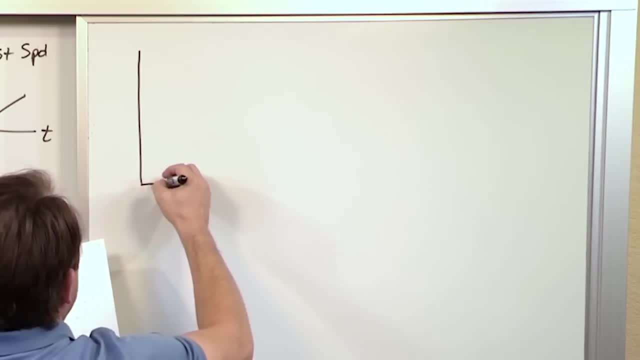 for instance, I'm going to redraw everything. I know it's kind of a pain, I'm going to have to redraw a lot of stuff here, but it's important. This section actually is one of the most important sections because it explains why limits are actually used. So this is time and distance. 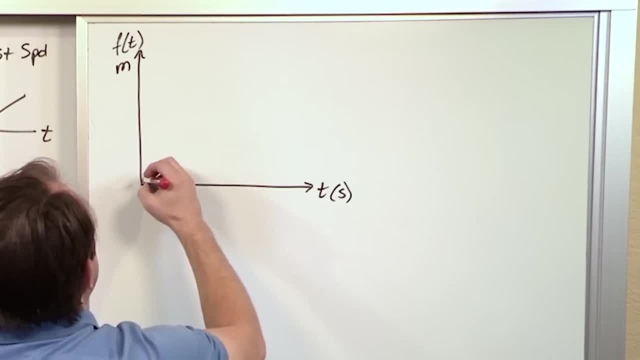 just like before, And I'm going to draw the same exact thing. So this is the function: rockets going up, as we already talked about. Now, if we wanted to figure out what the average velocity between two points is, we have to pick two points, So let's just pick some easy. 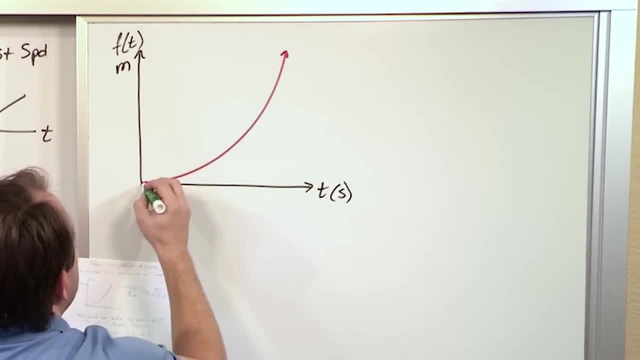 points. Let's try to figure out what the velocity of the thing is somewhere in here. So we could pick some time here and we can pick some time later here. Okay, The rockets obviously climbed in altitude here and we'll call this position one and we'll call this position two, Okay, So, 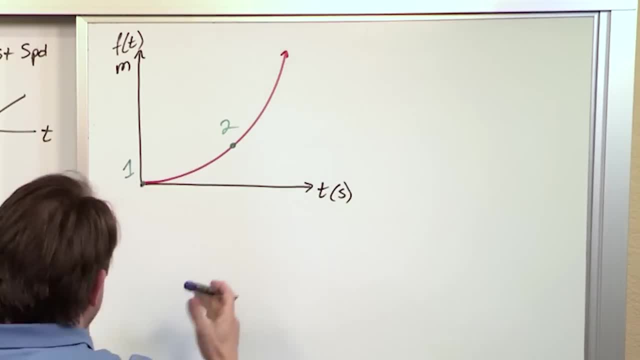 what we'll do. if we really want to figure out what the rough velocity is here, the average velocity. we'll say: average velocity Is equal to the distance traveled over the time. Okay, The distance traveled over the time. So what we end up doing then is when you, when you do that, what you're basically doing is you're. 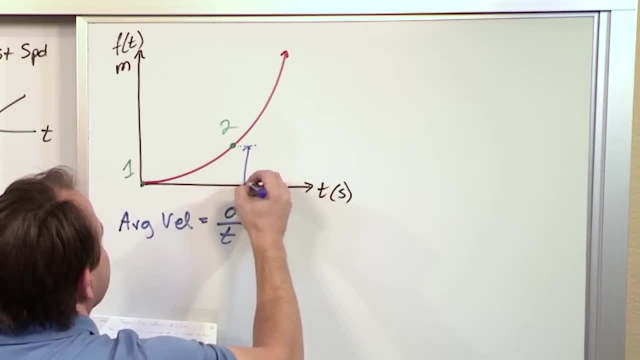 saying: what is the distance? This is the distance that the thing has flown up because, remember, this is meter. So this physical distance is the distance here. And then, if you look at this guy, this is the time traveled up until that point. So we start our stopwatch from here. We 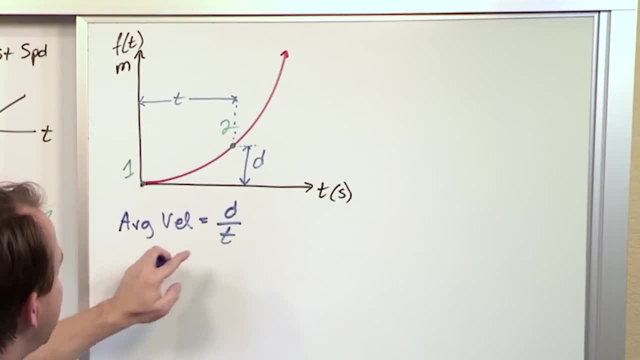 count how many seconds. We measure how high the thing has gotten in the atmosphere. We divide them, We get the average velocity. Okay, Great. Also notice that this forms kind of like a line here through these two points. I'll come back to that in just a second. Okay, Now let's move on a little bit later. Now we 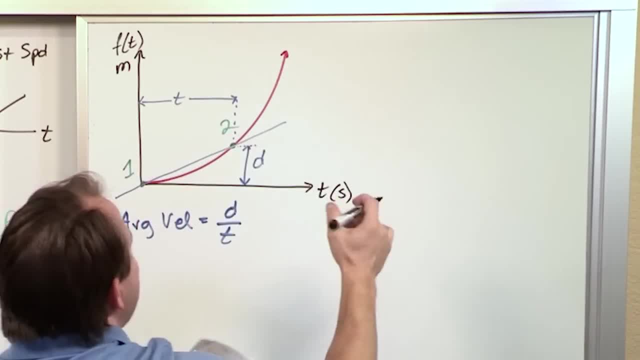 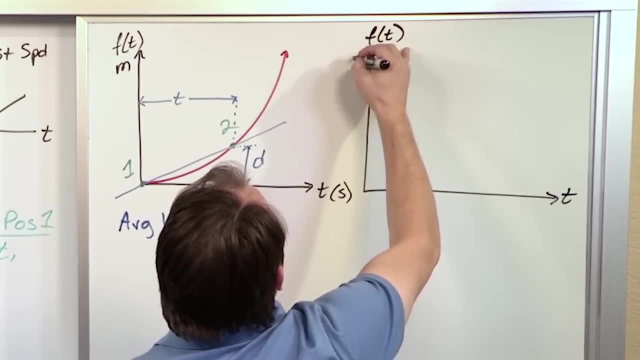 let the rocket climb up and let's say we want to figure out what the velocity is, as it's higher, it a little bit higher in the atmosphere. So let's draw another situation rather than just cluttering that up again. call it F of T. This is meters, So basically it's exactly the same The. 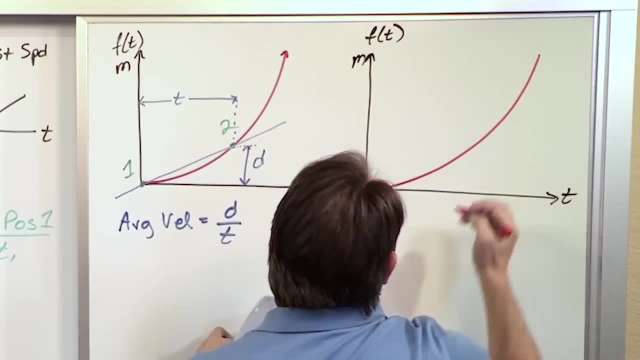 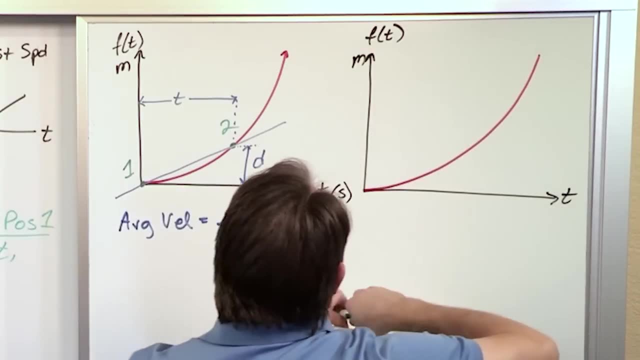 rocket has climbed its way up, on its way to orbit like that. All right. But now we don't want to know what the velocity is down here. We're interested in calculating what the velocity is maybe someplace farther up. So we pick some other points, We call this point one and we call this. 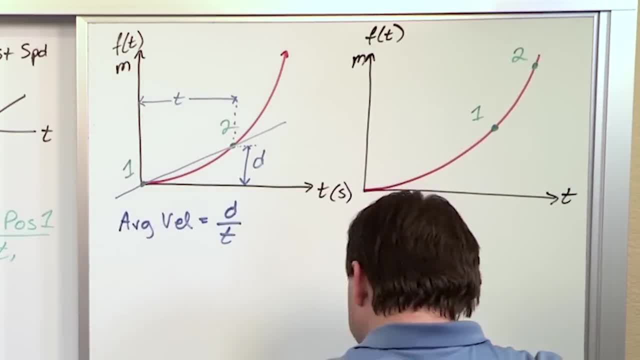 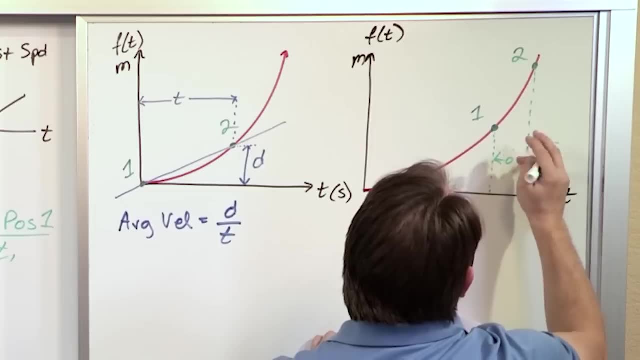 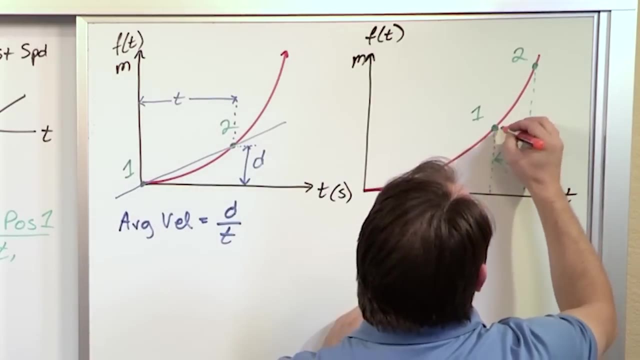 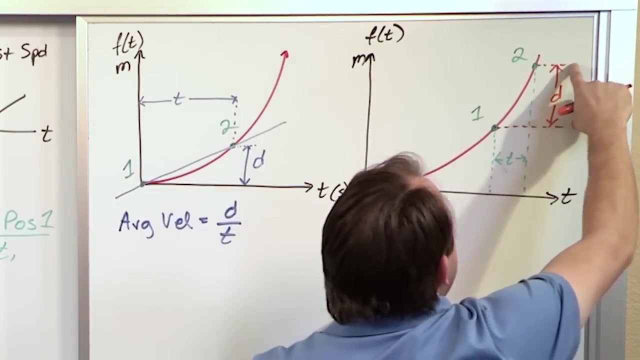 point two like this: Now, when you do this, you can see that this distance here, this is now the time Whoops, not D, This is the time to get there- And this distance right here, this physical distance measured in meters, is how high? 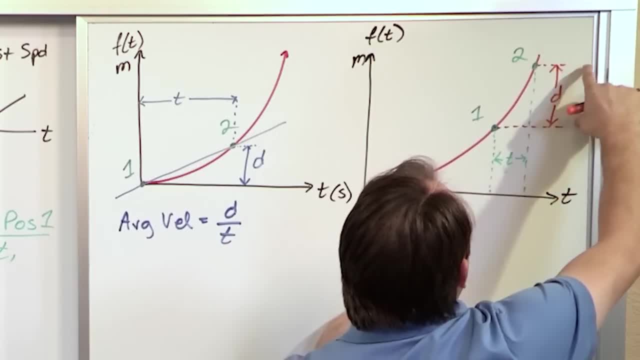 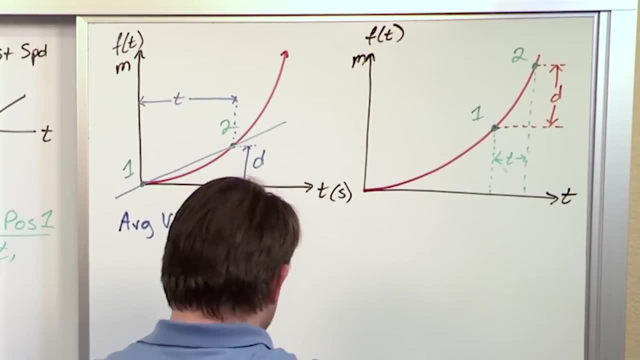 the rocket climbed right. So you can see it climbed an incredible amount, really, really high. Didn't really climb so much here, but it climbed an incredible amount over a relatively short period of time. So in order to calculate that velocity right there, we do the same thing. We say the. 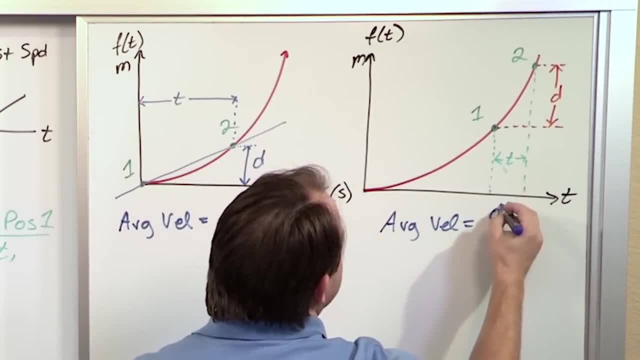 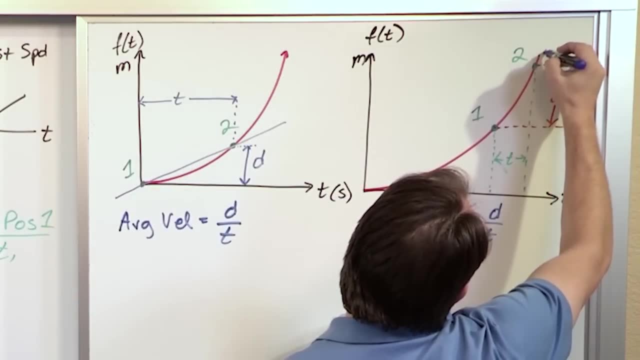 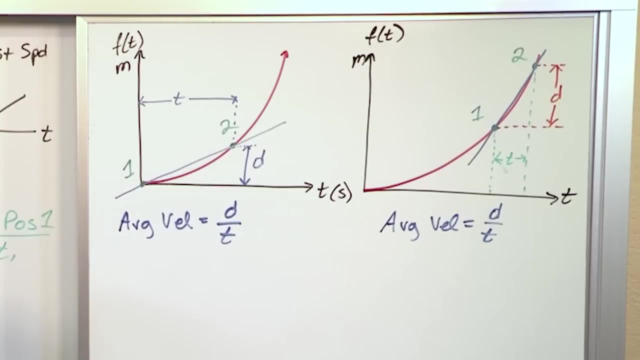 average. average velocity is distance over time. Okay, Same as before. And also notice that these two points, you can kind of draw a line through them as well, Something like that. Okay, So what do you notice from this? Well, we can already tell. 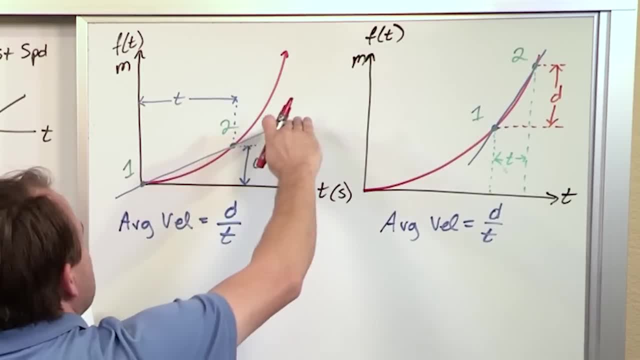 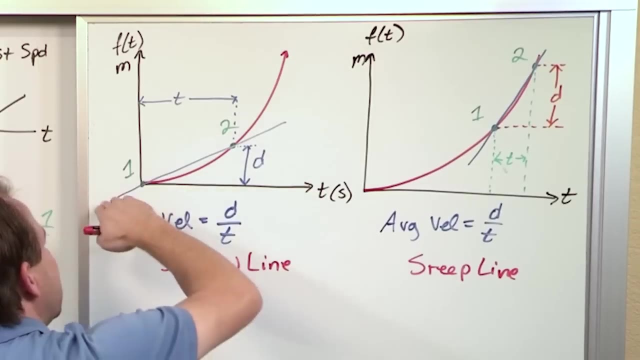 from before that this is basically a shallow line that connects these points And this is a very steep line here. So I'm going to say: shallow line connecting the points And this is a steep line that connects the points. So when you have a shallow line like this, what you're really doing is you're saying that you have a low. 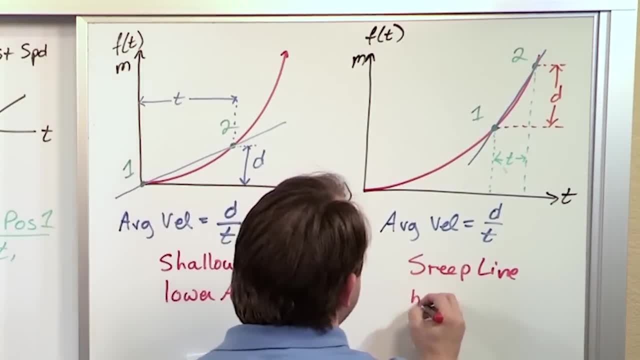 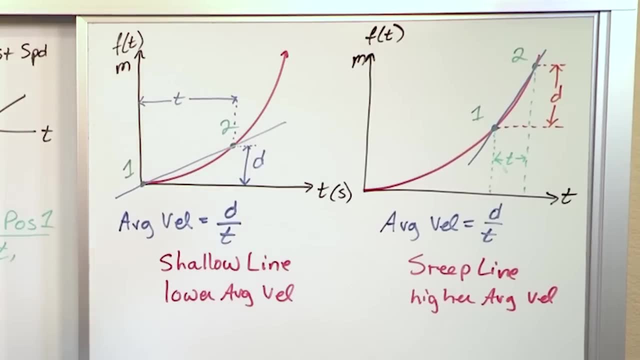 average velocity, and here you have a higher average velocity. Okay, So basically, these are very crude approximations. We want to figure out how fast or what the velocity of this rocket is. So if you're going to do it, you would have a stopwatch and you. 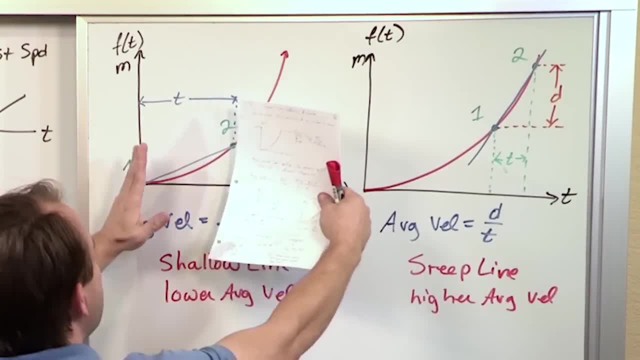 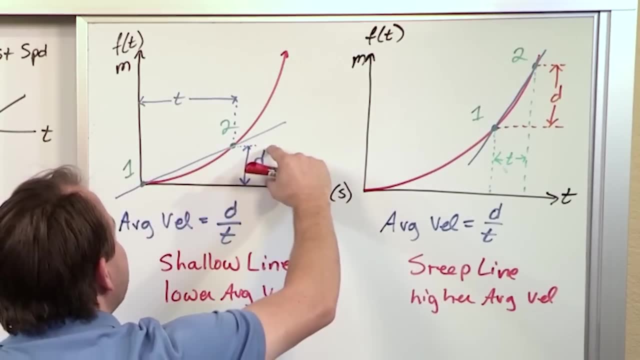 would measure everything right. So here we want to figure out what the rocket's doing roughly in here. So we picked two points and we figure out that it's roughly a shallow line. The reason it's shallow is because the rocket didn't rise very much. See the slope of this line, remember slope. 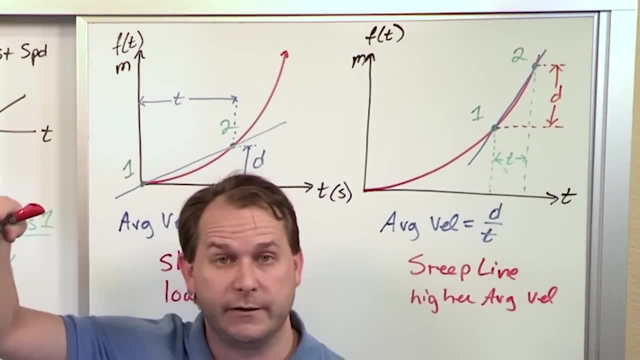 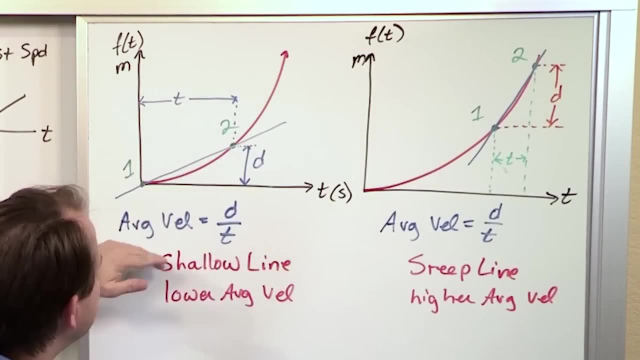 from geometry or slope from algebra. rise over run. If you rise a whole lot, then you're going to have a very steep line. But here we didn't rise a lot, We rise just a little bit. so we have a shallow line And that means we have a smaller average velocity. 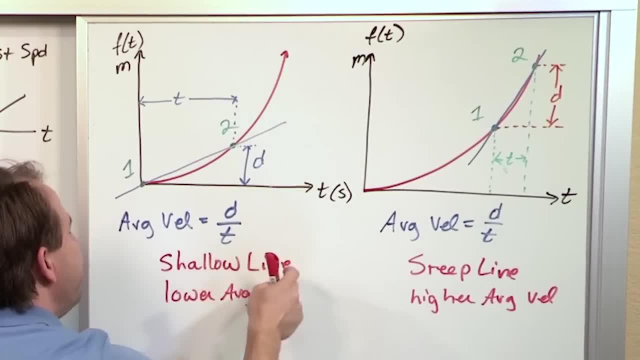 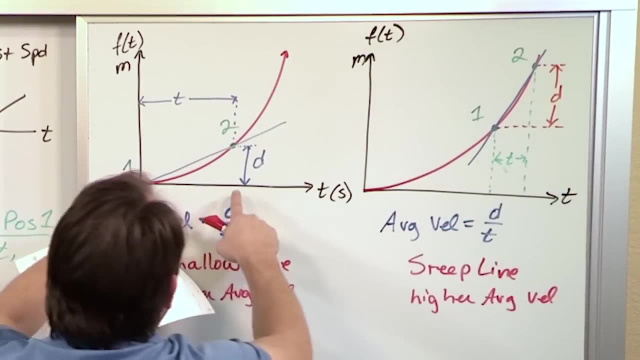 If you actually calculated the distance divided by the time, it will be a smaller number than here, because over here we climbed an incredible distance over a very short amount of time. Look at how much time we spent here. That's a long time. This is a little bitty time. 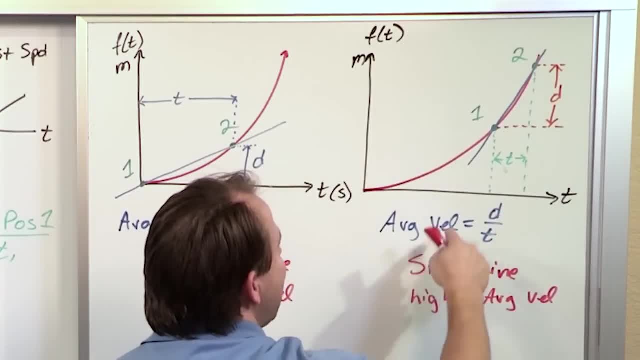 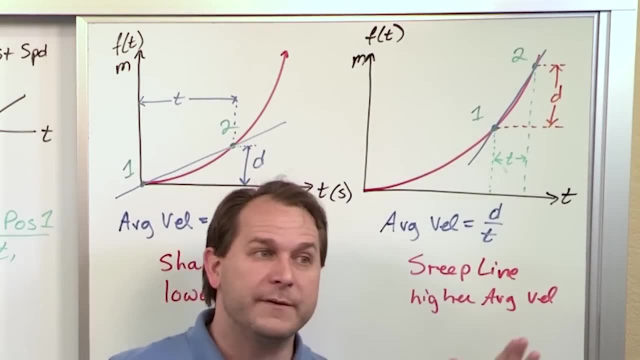 We covered a lot of distance, so the d over t is going to be higher and that means this line is steeper. I'm drawing this parallel because as you get more into calculus you're going to learn that the slope of the line tangent to a curve basically is its velocity, and that's what I'm. 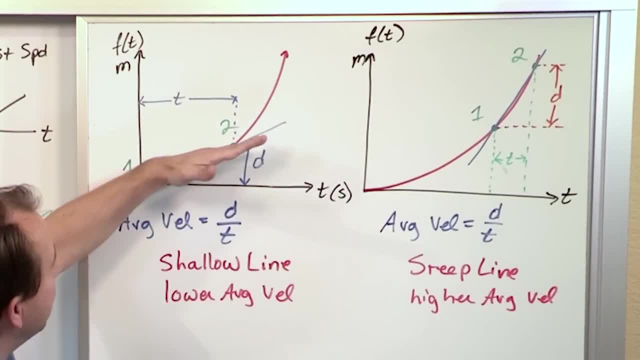 kind of trying to show you here. You know that the rocket's not very going very fast. here We have a shallow line. Here, you know, the rocket is going much faster and we have a steeper line. So the conclusion you can draw from this: the slope of the position. 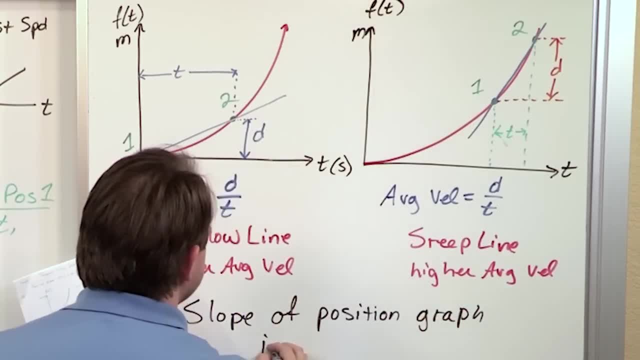 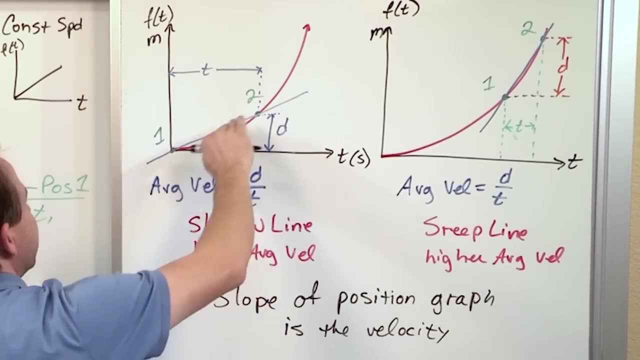 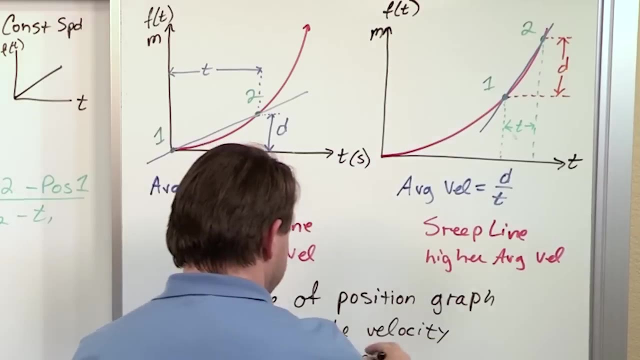 the position graph is the velocity. So see, we have very small slopes here, so the velocity is really small. Here we have very steep slopes. This is the position slope of the position here. so we have a very high or relatively higher velocity. But we're not done yet because we want. 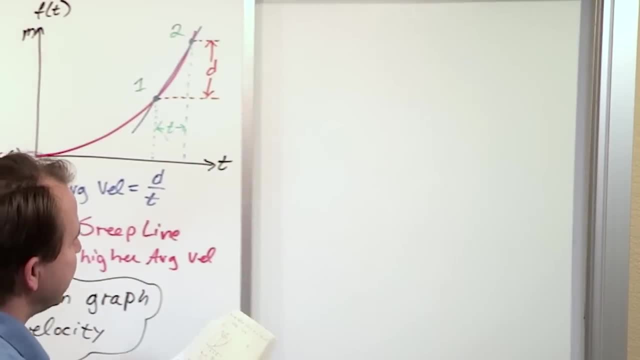 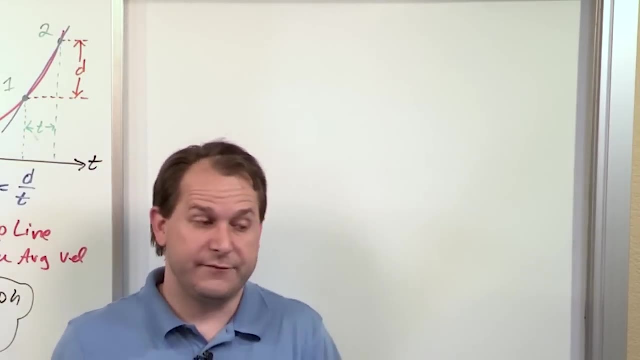 to apply limits to actually do this. So this is more of a conceptual thing. This is more of a concept Basically just saying: hey, if you're steeper, you're going to have a higher slope, You're going to have a higher velocity. If you're shallower, you're going to have a lower slope. 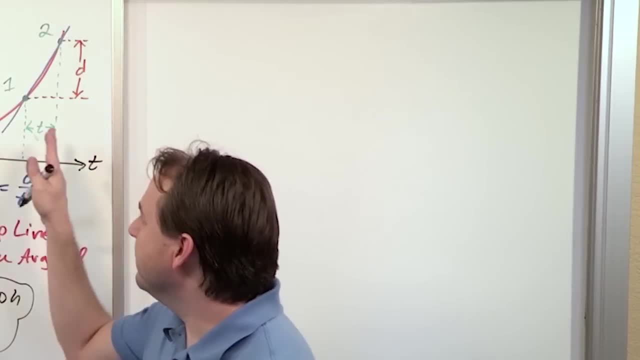 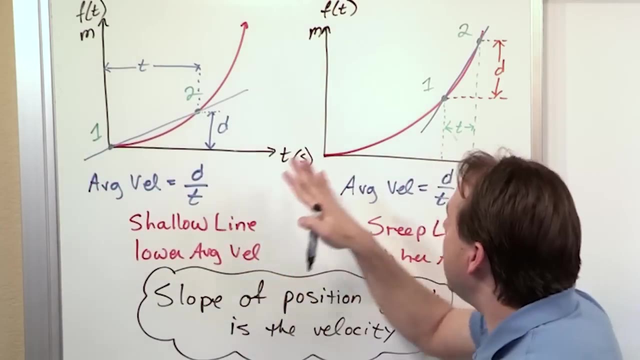 You're going to have a lower velocity. But the problem with this, doing it this way, basically, is that you see, this is kind of a representative velocity in this part of the equation. So you're going to have a higher velocity in the trajectory, That's true, And this is kind of a representative. 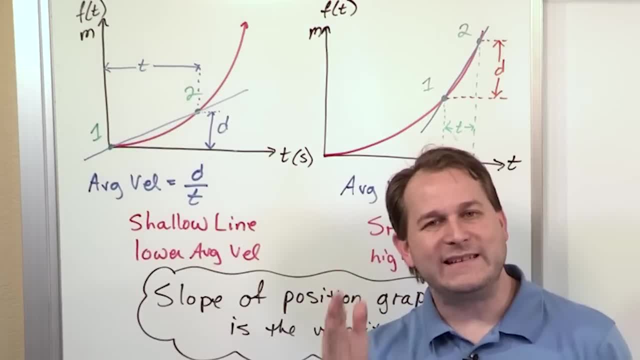 velocity in this part of the trajectory. But in calculus we don't want to find an average like that, We want to find the exact velocity. If this rocket is a very expensive rocket, I'm sure it has some speedometer there that's telling you how fast it's going at every single moment in time. 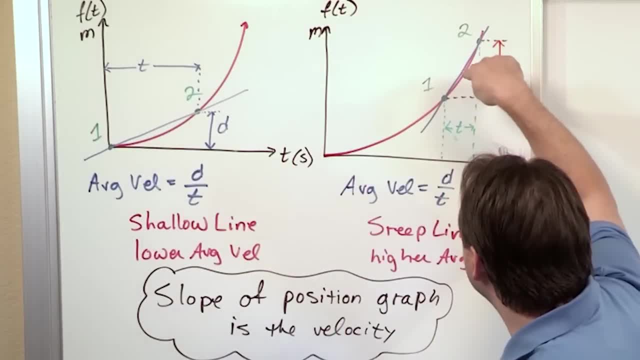 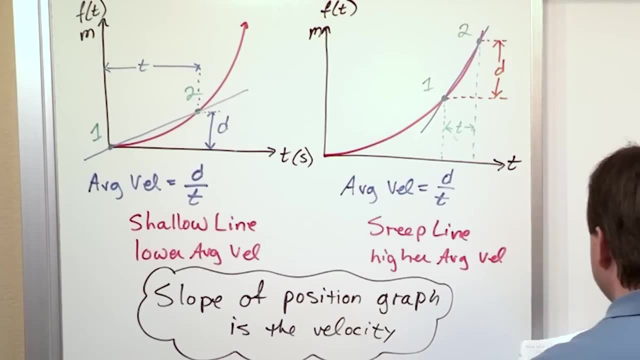 We don't want to just look between these two points and come up with an average. We want to know exactly how fast it's going right here, Don't you think? when we build rockets, we really want to know that. Okay, so we want to figure that out. We can use calculus to do that, And that's what we're. 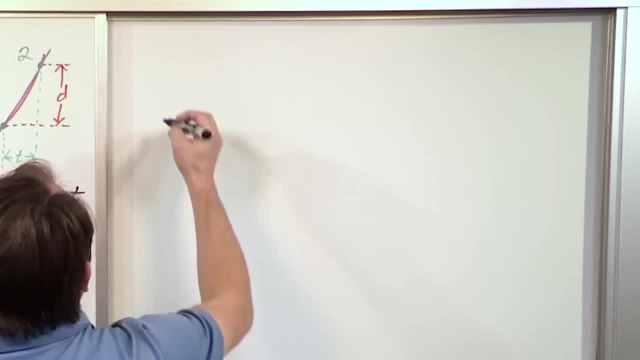 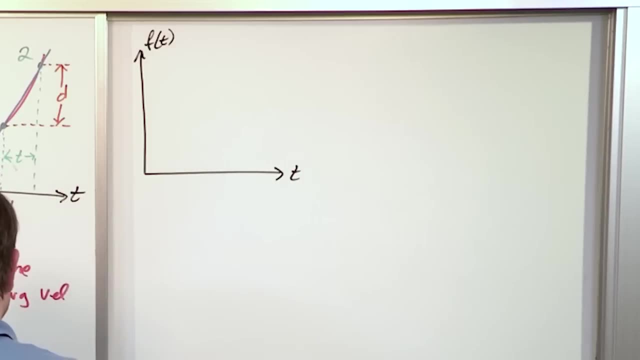 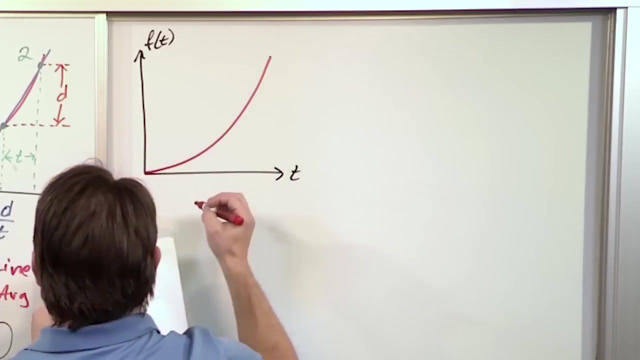 going to do. That's why we use limits. So let me again draw everything again. I know I'm drawing a lot, but I promise it's important to do to make sure you understand this guy. Okay, so we're going to draw our nice function again, But this time we're going to put some numbers here. We'll say: 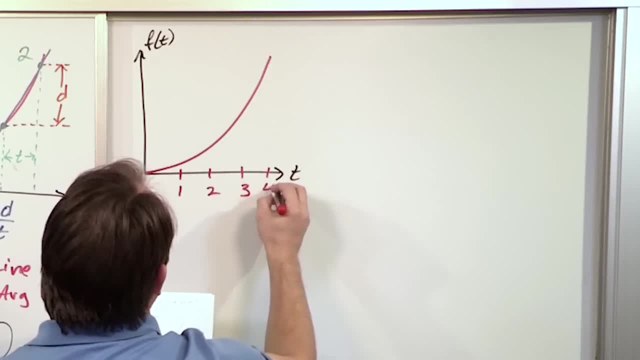 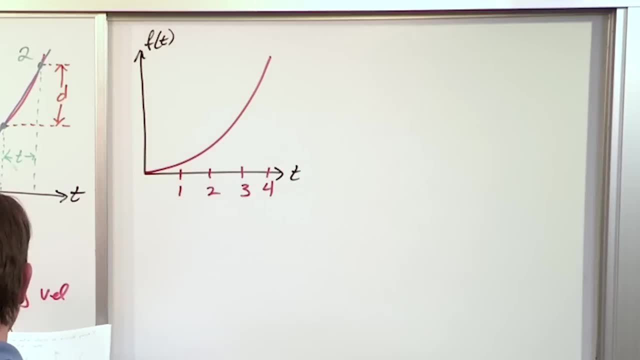 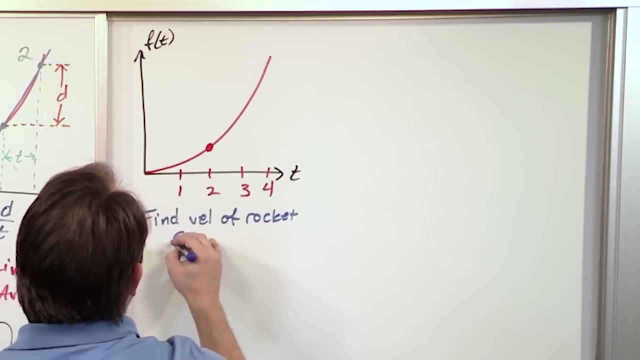 one, two, three, four seconds. Okay, and let's say we want to find the velocity at this point, Right here, at t is equal to two. So we want to find the velocity of rocket at t is equal to two seconds. We don't want to know what the velocity. 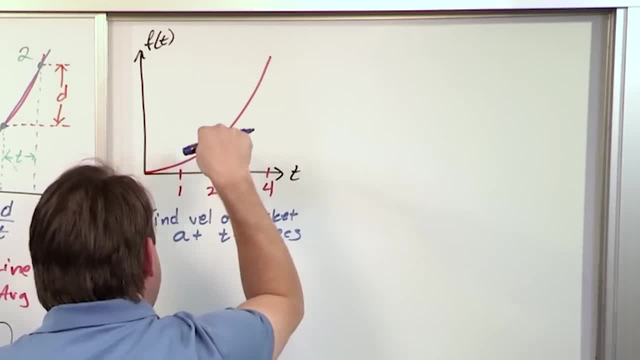 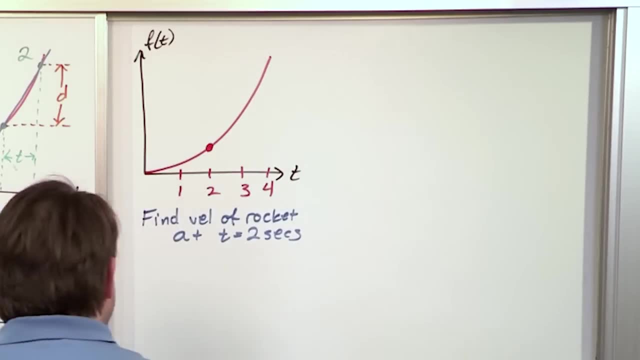 is here. We don't want to know what the velocity is here, We want to know what is right at that point. So how would we do it? Well, we do what we've already been talking about doing: We find an approximation for it and we go from there. So let's just say that we 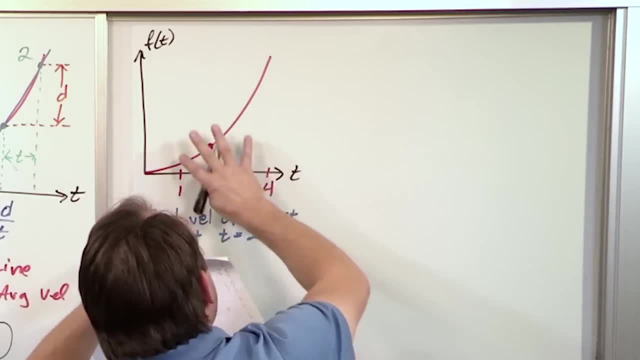 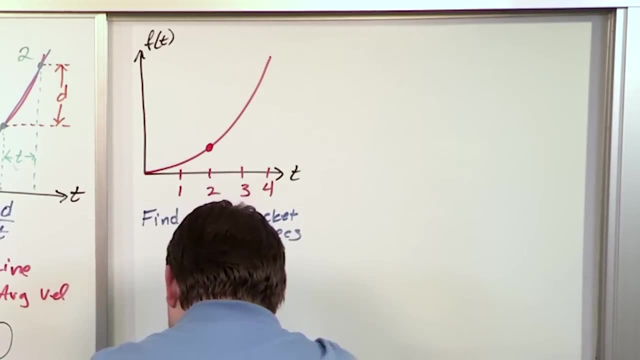 we don't quite know yet how to figure out what it is there, but we know how to get kind of a representative. So let's just look between these two points. Here is that t is equal to two. Let's go up and look at: t is equal to four. Let me extend this graph up a little bit. 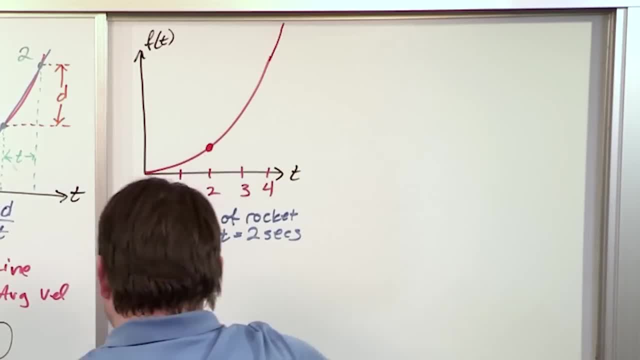 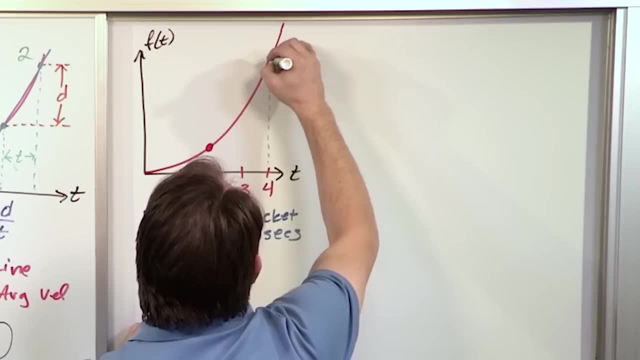 just to make sure nobody gets confused. So we'll go up like that, whatever. And then we want to look at: t is equal to four. So if we follow this guy up here like this, it's right at that point. And again, we already know that this forms kind of like a line like so: 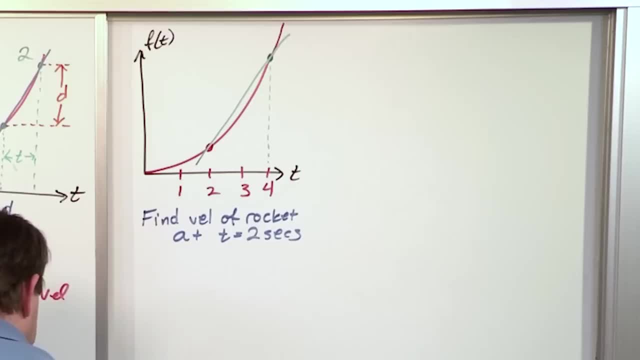 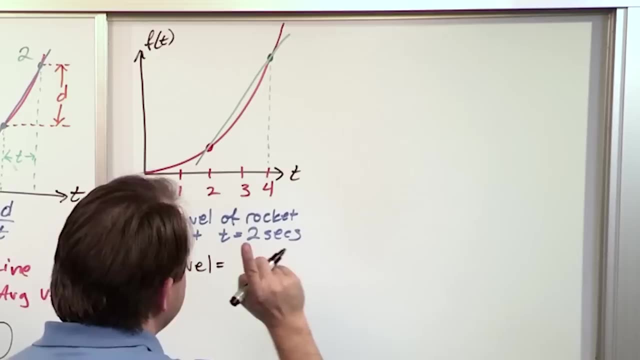 So we want to figure out what the velocity is at this point. So the way you do that is, you say the average, the velocity, which is kind of what we just did a second ago. But here's how we're going to start to put numbers into it, Because before I was just drawing pictures, Here we're. 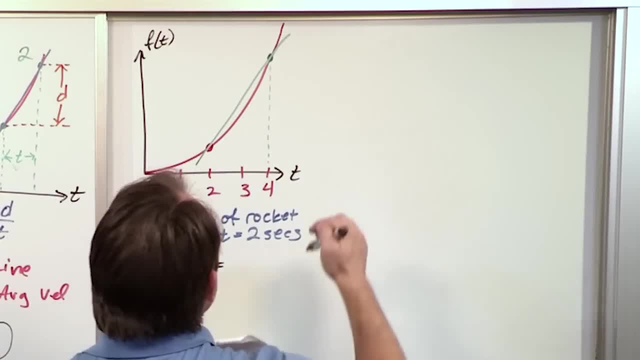 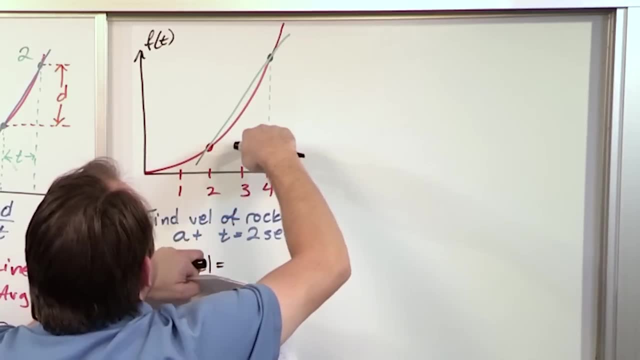 going to actually do it, as if you were going to actually do it. You want to find the distance, because it's distance over time. right, The distance here? The distance here is this point on the curve minus this point on the curve. So you want to subtract the distances here. So what you do, 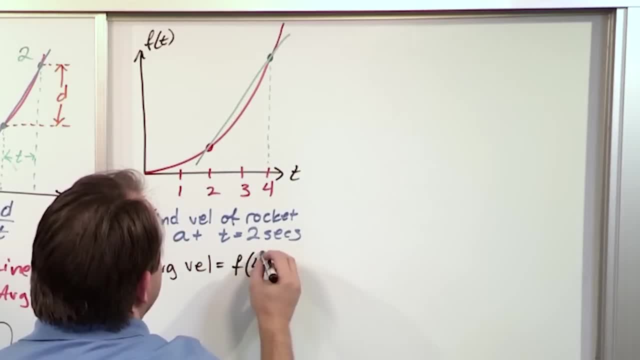 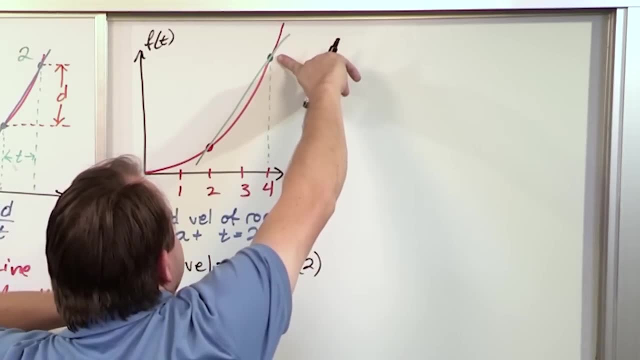 is you say the function here evaluated at four seconds, minus the function here evaluated at two seconds. This is going to give you the vertical distance, because f of four. this is how high the rocket is at four seconds. This is how high the rocket is at two seconds. You subtract them, you 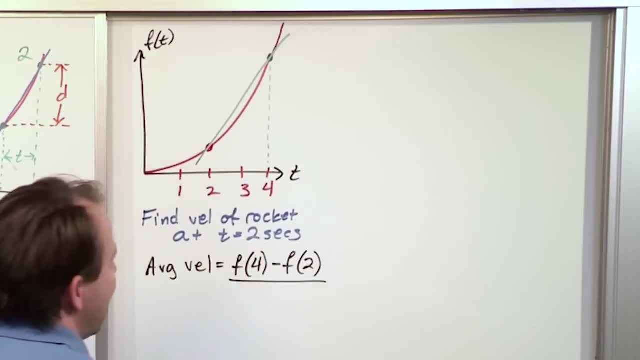 get the distance there, And then you want to divide by the time it takes to do that, which is four minus two, So two seconds. you know, going from here to here is two seconds. four minus two. Okay, so the average velocity at t is equal to two seconds, would be given by this formula. Okay, now let's move over here. 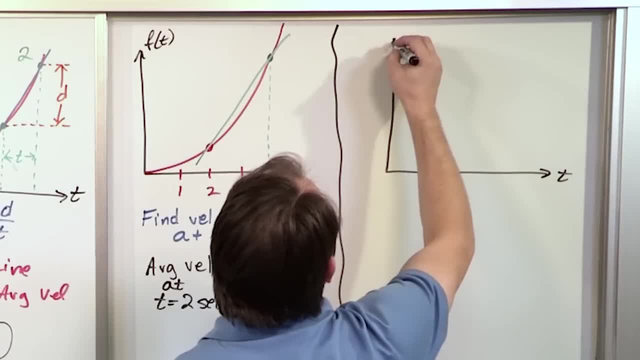 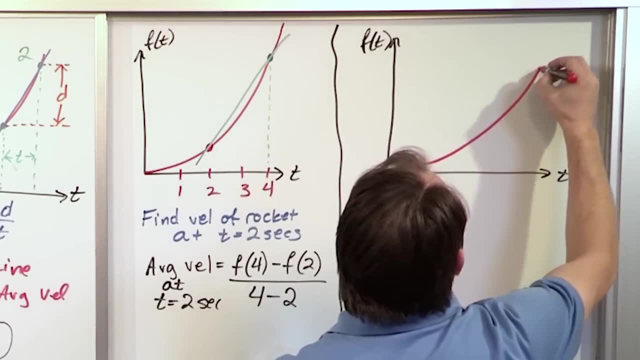 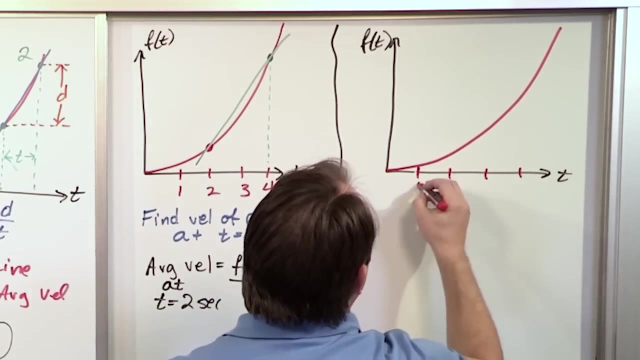 and draw the whole thing again. So here's t, here's f of t, and then we're going to draw the whole thing again. It's not going to be exactly the same. I'm going to try my best and I'll speed up just a touch because we can. So one, two, three, four, one. 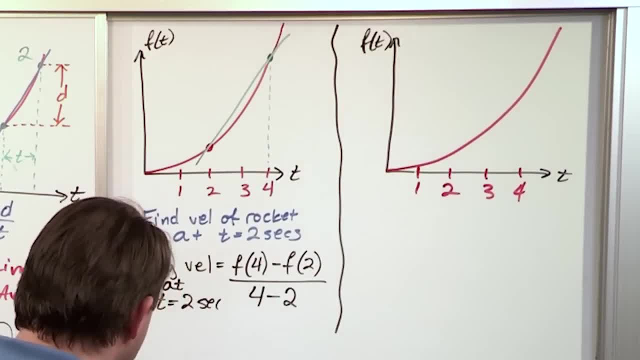 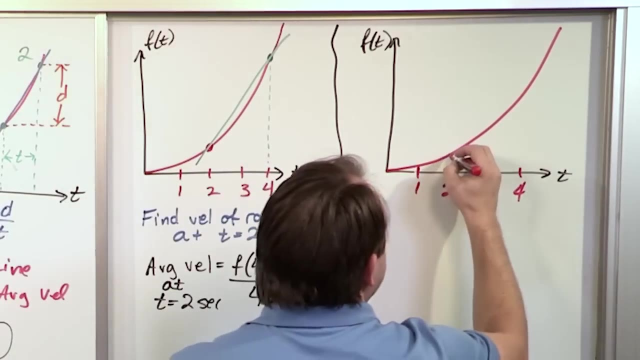 two, three, four And over here. what we want to figure out is we want to know what the velocity is at this point. So we start with a very crude approximation, drawing a line through these two points. But if we wanted a more accurate representation of the velocity at that point, which is at this, 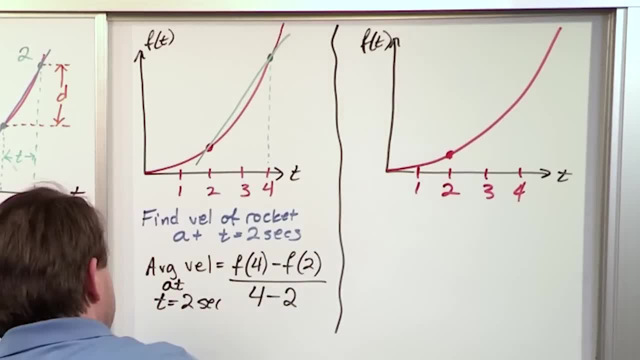 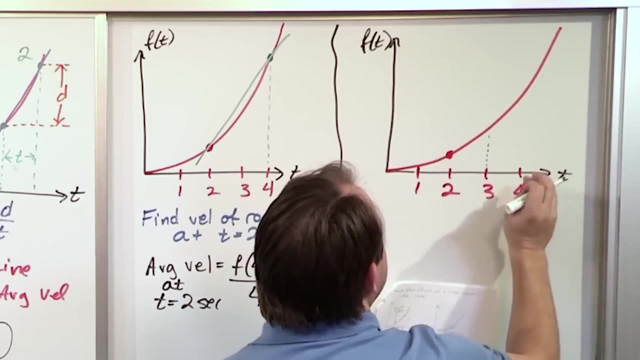 point right here, then maybe we wouldn't choose a point so far away. Maybe we have some really good fast computers, so we want to do it maybe a little bit closer. So we, instead of going way over here to t is equal to four, we go here. Okay, so we can get a slightly more accurate a. 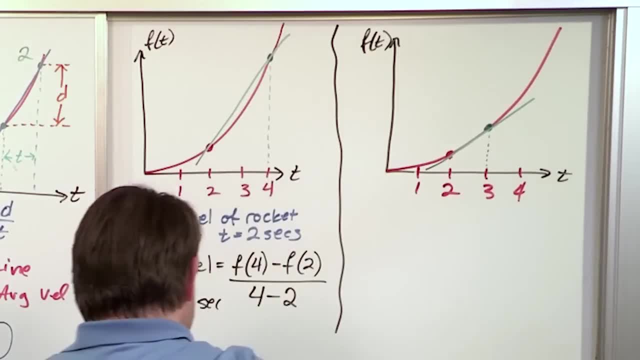 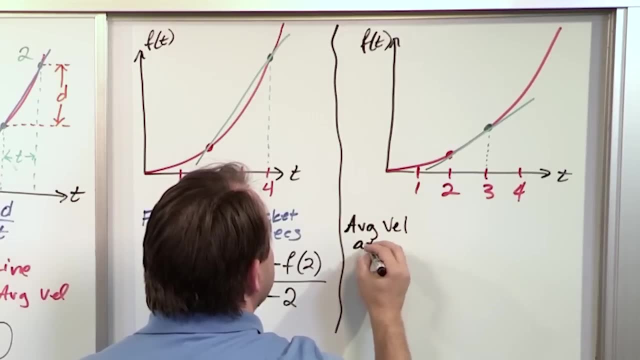 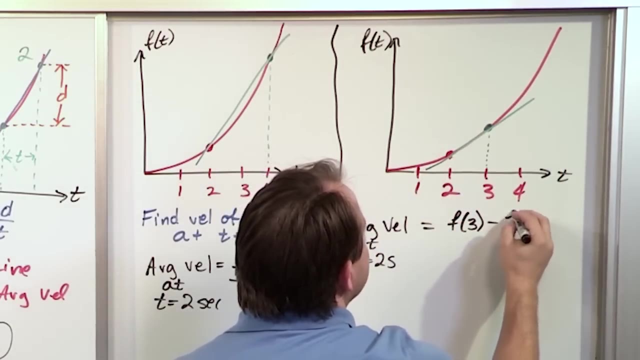 approximation for the velocity of the rocket at this red point here by drawing a line between those two guys. And then the way we figure it out- the average velocity at t is equal to two seconds- is the vertical distance which is f of three minus f of two. This is the distance, It's the 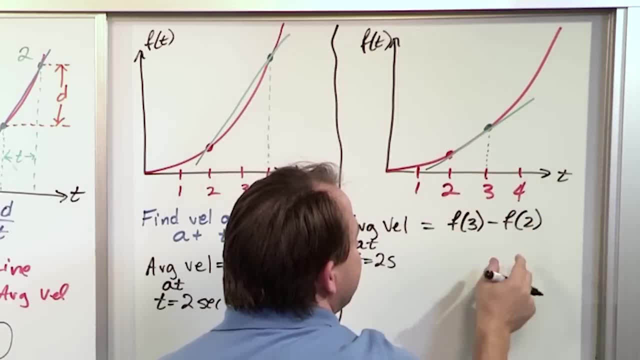 height here minus the height here, Height at t is equal to three. Height at t is equal to two. Subtract them And then the time it takes. You know it's taking one second, Three minus two. Notice what's happening here. So we can get a very crude approximation by drawing one of these. 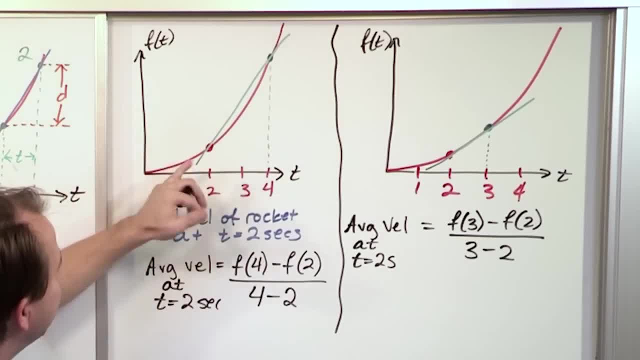 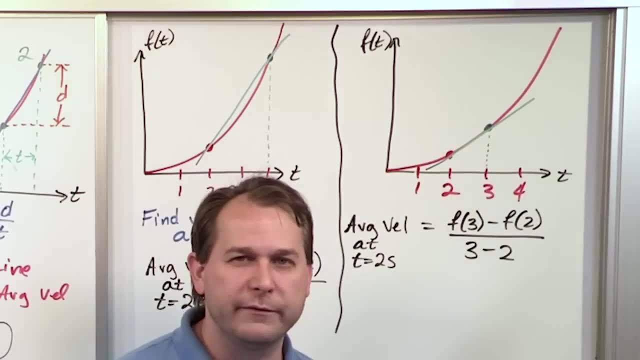 weird lines through the point. we care about and averaging it over a long period of time. But then we can get a slightly more accurate representation by choosing the point a little bit closer to the point of interest. So you see what's happening here. We can make this closer. 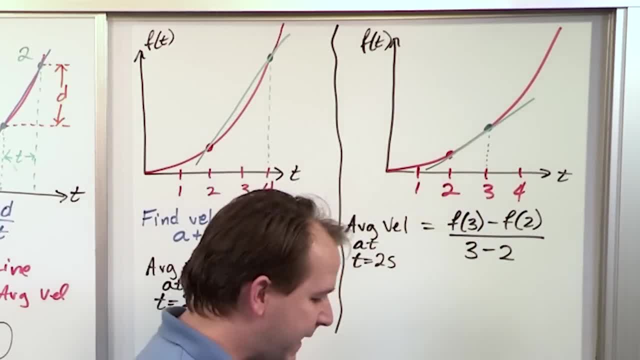 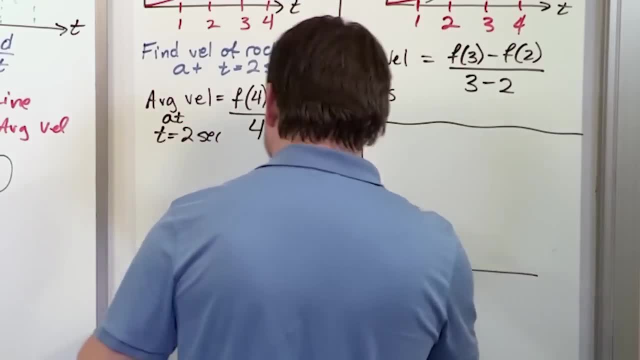 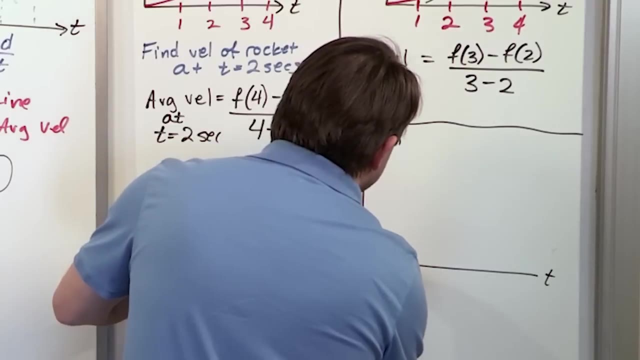 and closer, and closer and closer to the point that we actually care about. In fact, we'll draw one more for you here. Let's go and choose something a little bit closer. even So, this is f of t and this is t. We can go over here and draw the same guy here. 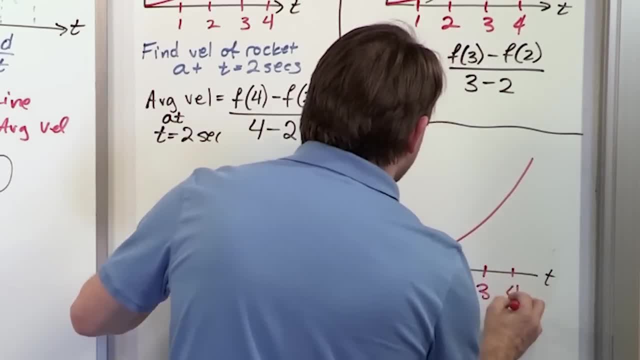 One, two, three, four. One, two, three, four. And, don't forget, we want to know what the velocity is at. t is equal to two, which is right there. So instead of, like we did, up here looking at 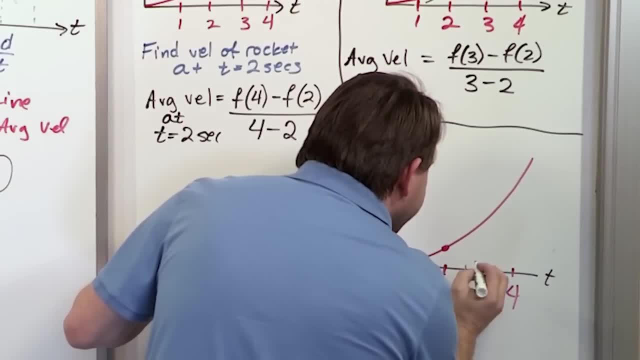 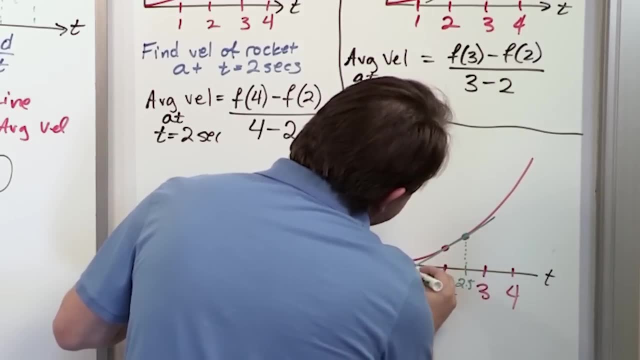 three seconds and drawing a line through there. maybe we go to two and a half seconds here, 2.5.. We go up, We find this point right here And then we draw a line through these guys. So you see, I'm making it closer and closer and closer. And in this case, 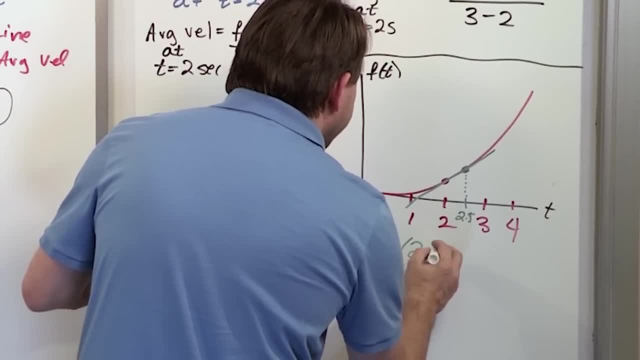 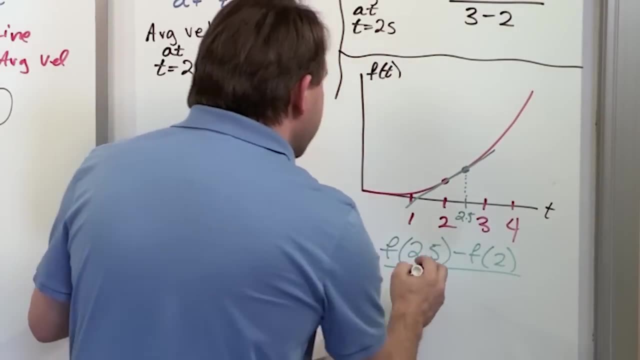 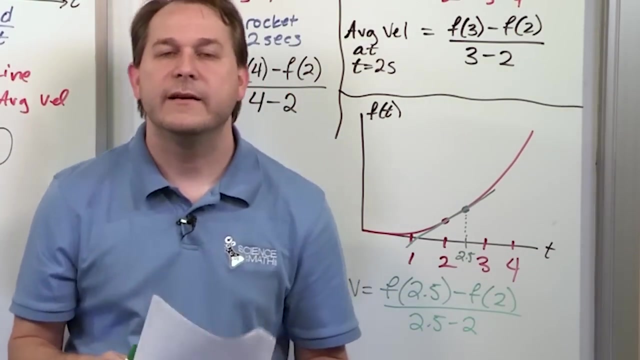 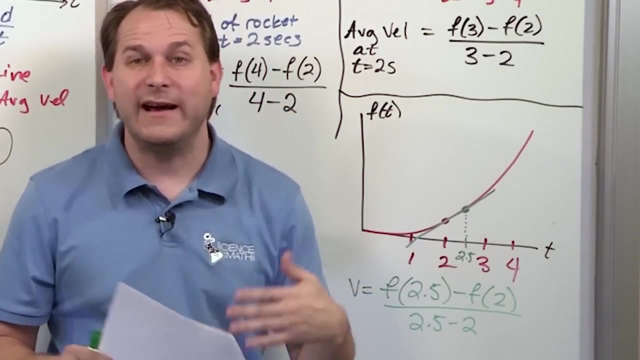 the velocity is f, 2.5 minus f at two seconds- This is the vertical height between these guys- that the rocket climbed- 2.5 minus two. So you notice that in limit theory I was very careful to tell you that you don't ever actually get to the point when x approaches zero. 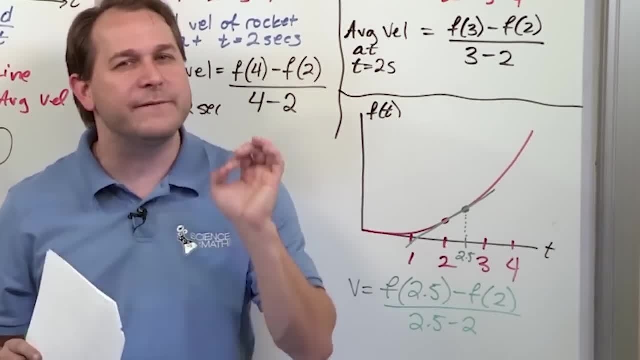 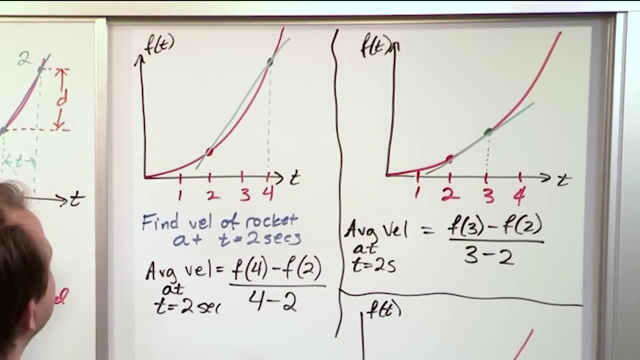 x approaches one or x approaches pi, You don't ever get there. You just get infinitely close. And so we're presented with the same problem here: We want to find the instantaneous velocity. At first you'll look at it and say it's impossible because everything's changing. Well then you say: 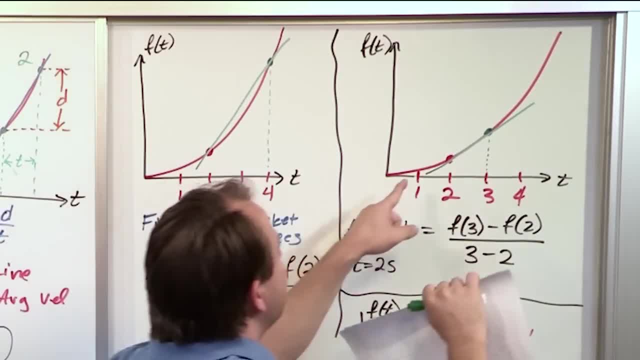 okay, I'm going to find this average. That's going to be my first guess. And then you go over here and you say, well, I'm just going to pick a point a little bit closer and say, well, I'm going to. 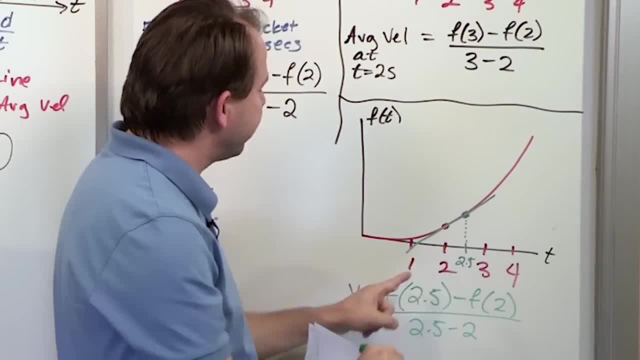 choose this average. This is a better guess. And then I'm going to get even closer and closer, And then I'm going to get even closer, And then I'm going to get even closer, And then I'm going to get closer And I'm going to say: this is a really good guess. Well, what would happen if you kept? 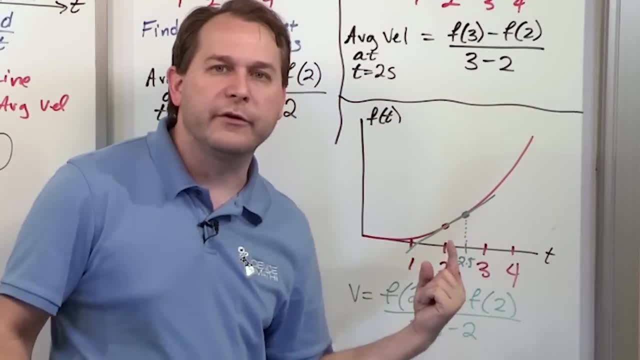 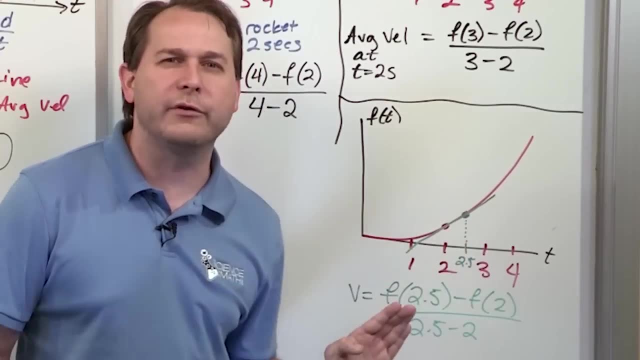 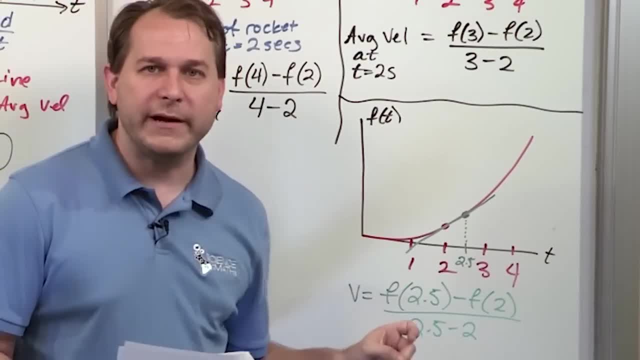 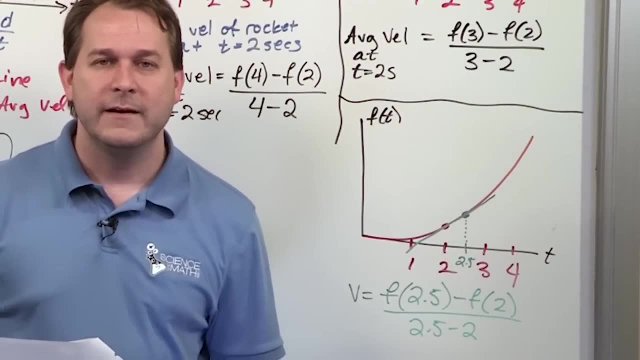 infinitely close answer to the velocity at this point. And we use a limit to do that, because limits is the thing that we use in math to get infinitely close to something. Let that sink in for a minute. Play that a few times, because that's exactly what limits are. 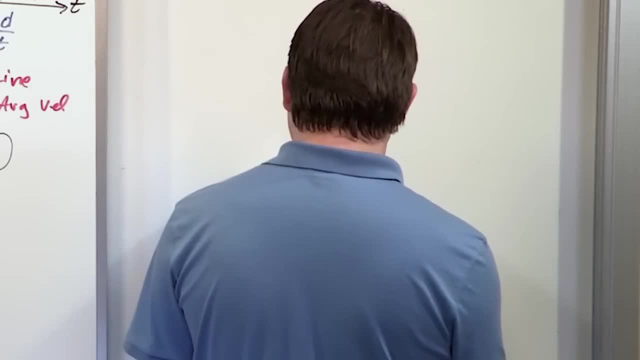 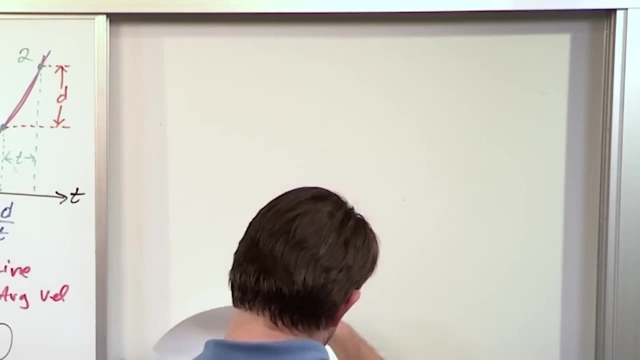 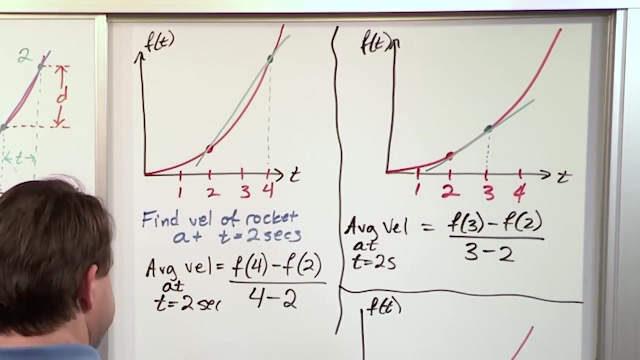 used for Exactly what limits are useful for. All right, So, for instance, okay, for instance, well, let me see here, Let me stay here on this board here. I hate cluttering up a board like this, But you see, 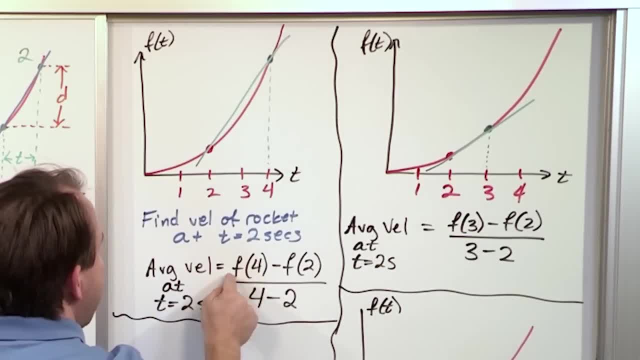 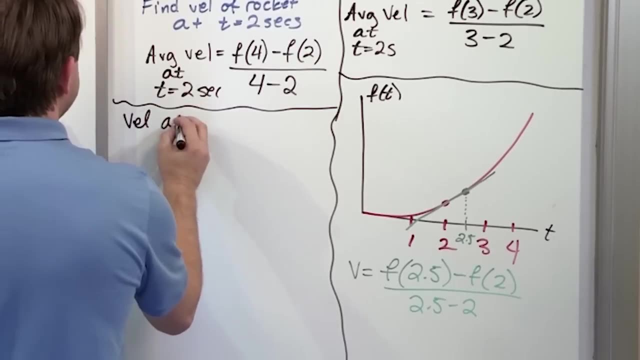 here we found the average velocity Between these two points. it was f of the right-hand point minus f of the point we care about, divided by the right-hand point in time minus the point we care about in time. So the way you generalize this, okay. if we wanted to find the velocity at, t is equal to two seconds. 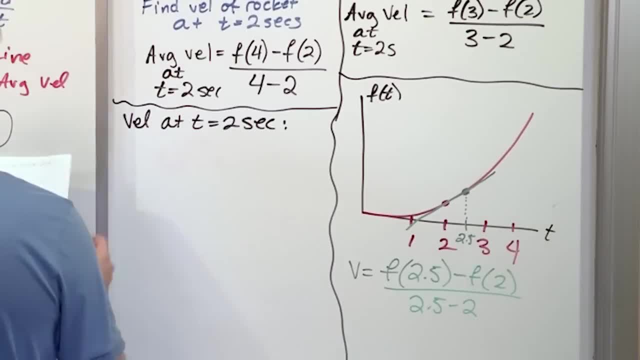 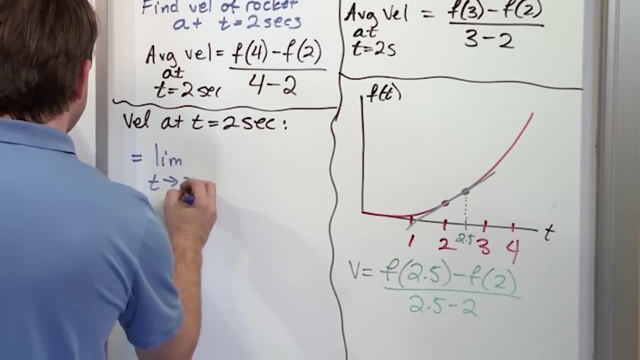 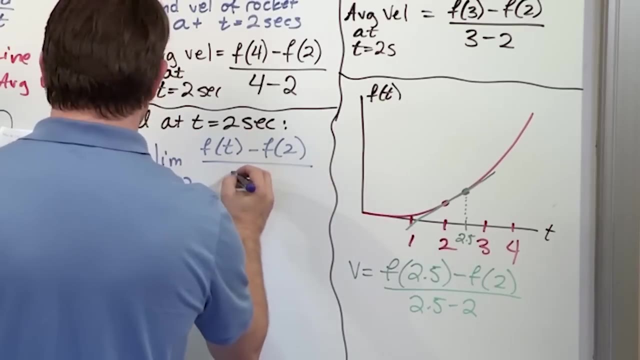 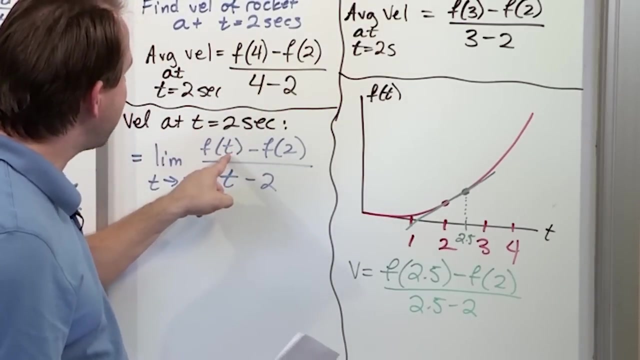 the way that we would do it is we would say: the velocity is equal to the limit, as t goes to two seconds. Okay, So f of t minus f of two over t minus two. Make sure you understand what's happening here, because what's going on is: it's the same subtraction on the top, but now we put a variable in here. 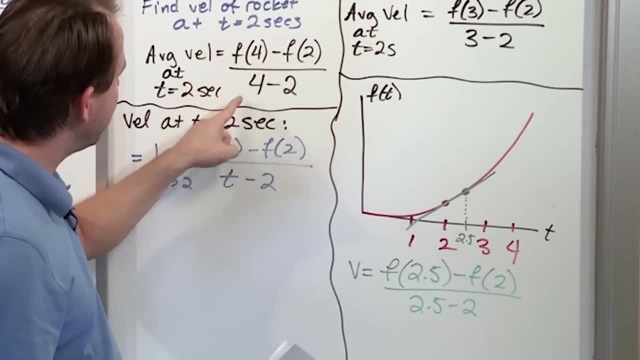 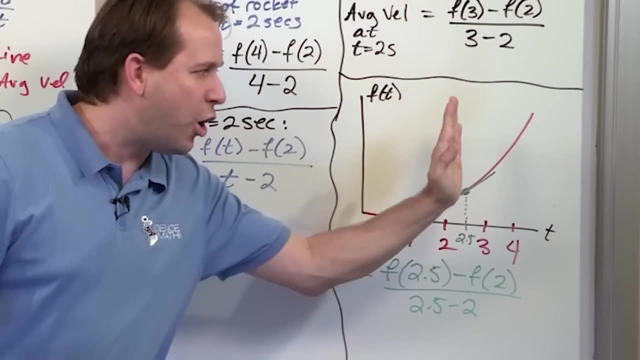 because this can be anything, And in the same place, on the top and bottom, where that right-hand time is, we just replace it with a variable. But this variable gets really, really, really close to the point of interest. All we're doing when we do this calculation is we're arbitrarily sliding. 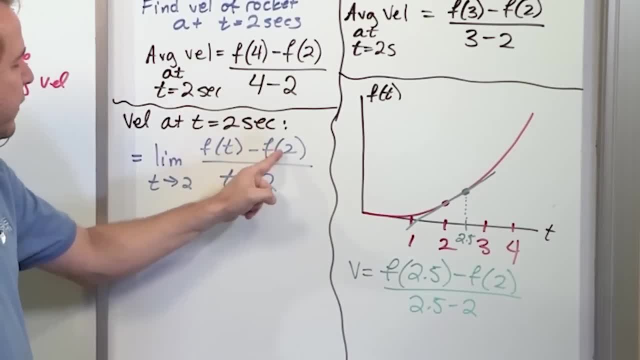 closer and closer to the point of interest. So we're going to be doing this calculation. and we're going to be doing this calculation is we're arbitrarily sliding closer and closer to the point of interest, closer to the point we care about. taking the difference in the rocket's height between 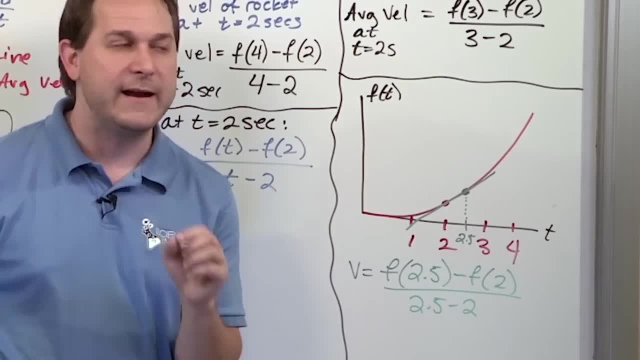 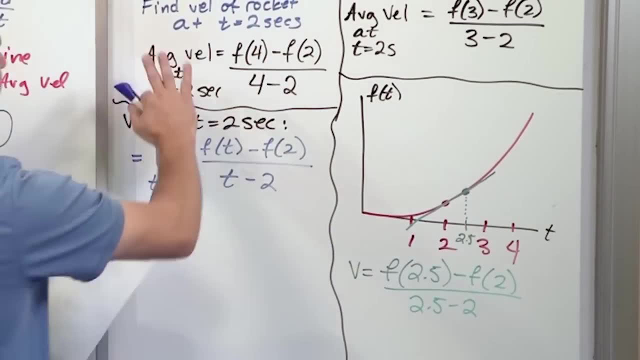 those two points and then dividing by the teeny-weeny-weeny time it took to do that. Basically, we're taking and we're sliding these points infinitely closer together doing this calculation. Now, this was written in terms of this problem, where t is equal to. 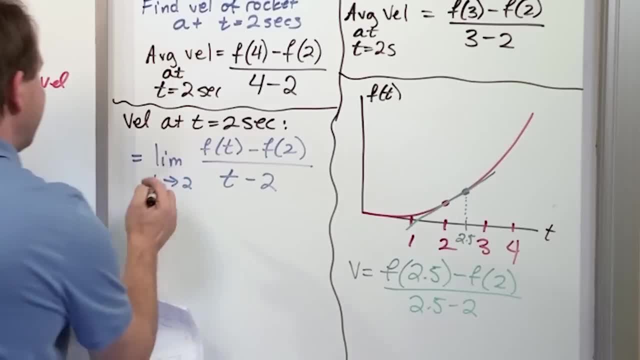 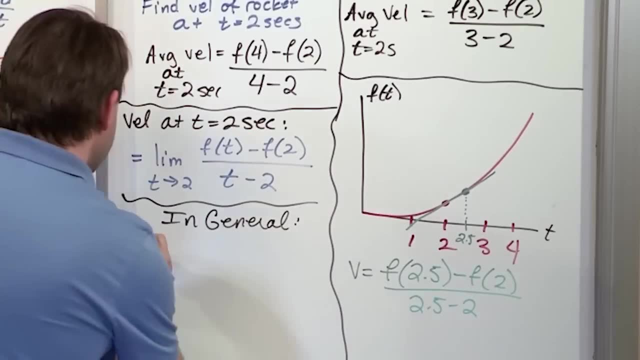 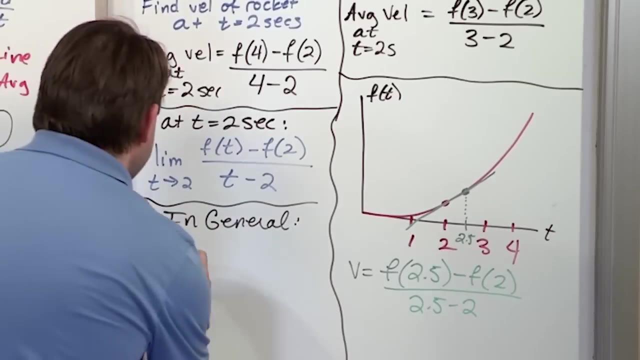 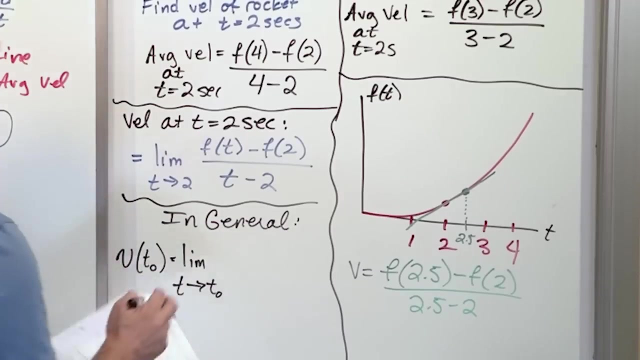 two seconds. okay, Where t is equal to two seconds, But in general, this is what you're going to see written in your book. The velocity at some point in time, t0,, the instantaneous velocity at some point called t0, is equal to the limit as t approaches: t0 of f of t minus f of t0. 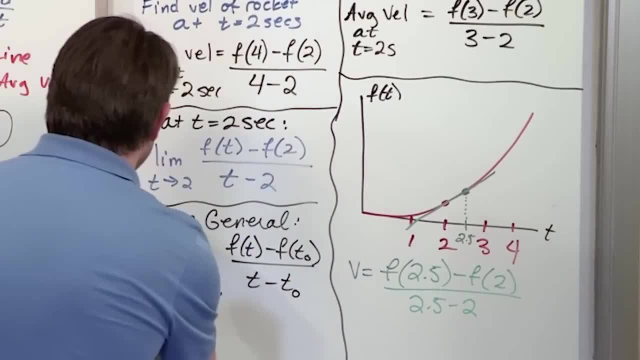 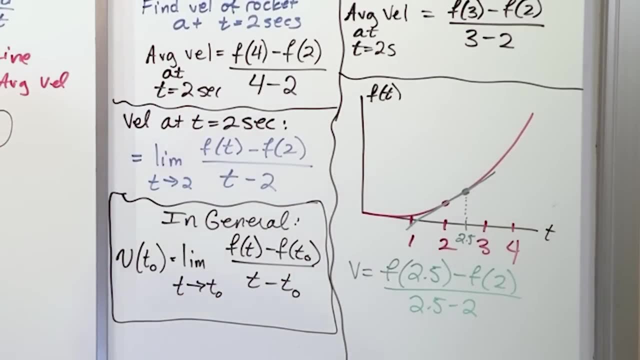 over t minus t0.. And this is so important, I'm actually going to circle it. I don't circle too many things, but I circle That one because that's really important. Now, what does this mean? This is basically. 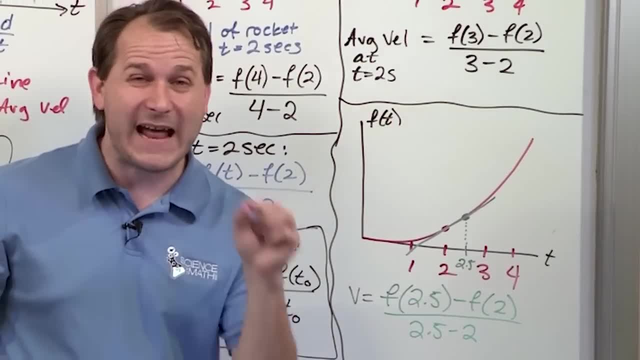 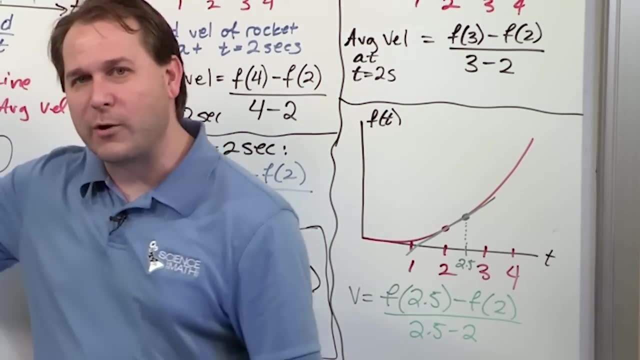 telling you how to find the velocity of a rocket at a specific point in time, even though the velocity is constantly changing. right? So we go from the kindergarten problems or the fourth grade problems, where everything's constant, everything's easy, to the calculus. 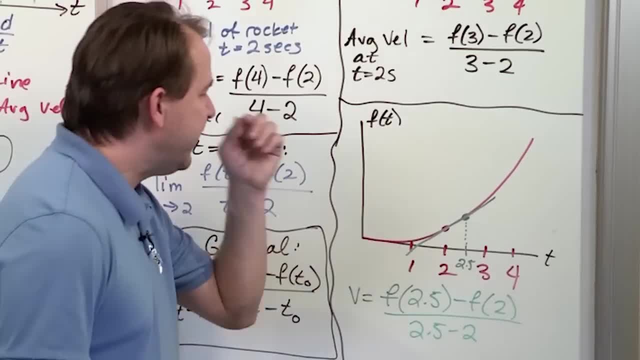 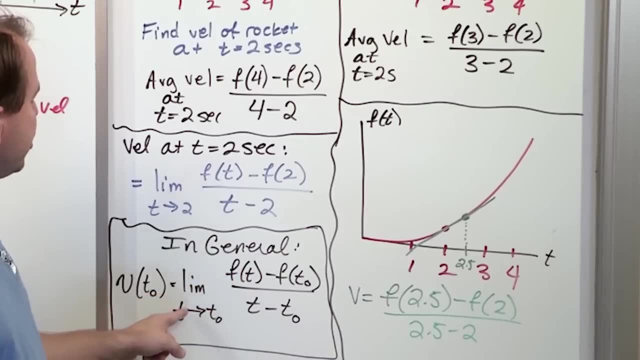 problems where we have to use a limit because everything is changing. So what you would do in practice is you would figure out whatever the function in time is okay And then you would subtract. You would subtract off the function in time where I care about. That's giving me the difference. 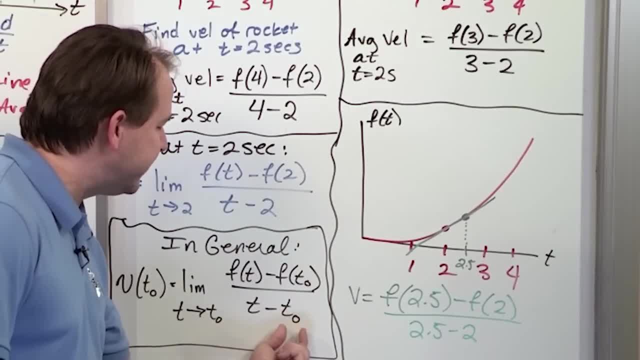 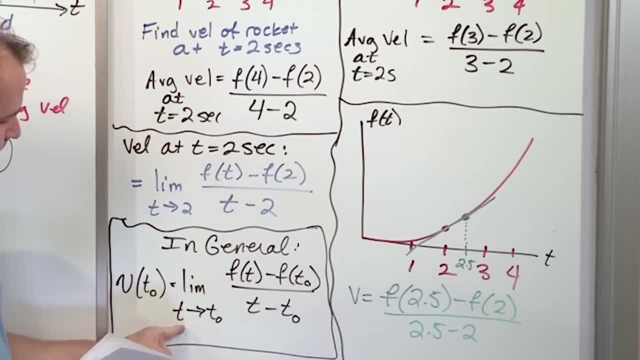 in the height. This is giving me the difference in time between the point I care about and the point that I have there, And I slide that point infinitely close, continuing to calculate and making t go to t0. Now I think this whole thing is going to be a whole lot more easy. 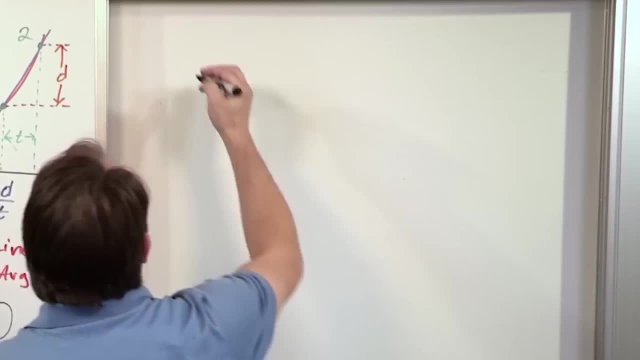 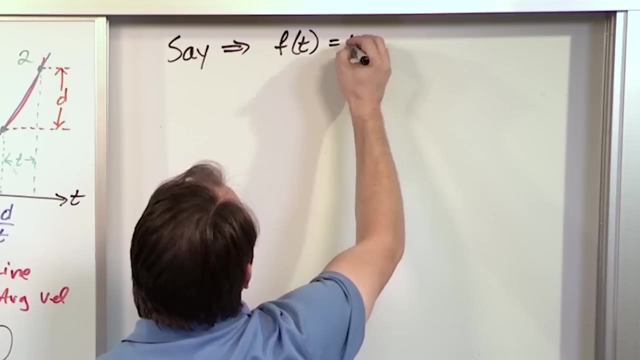 for you to understand if I get a real problem to you. So let's say that we have a real rocket in the function of time, which is the height, which is the function of time, is just t squared. okay, t squared, which is a parabolic. 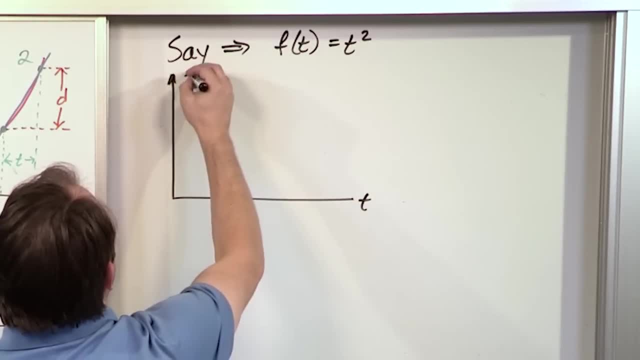 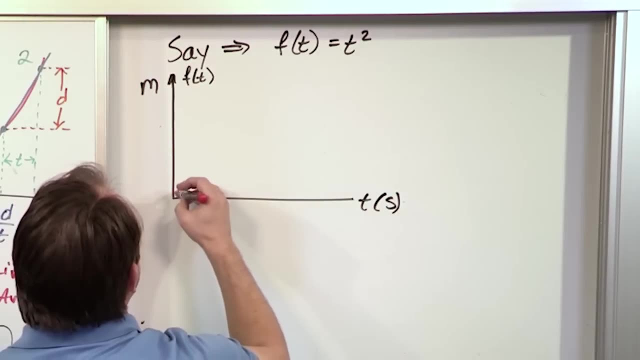 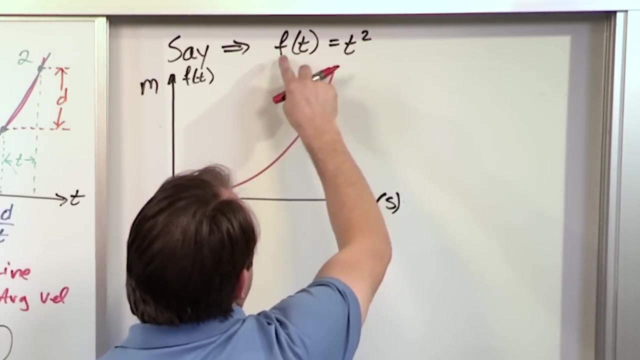 kind of thing. okay, So here's t, here's f of t, and this is in meters and this is in seconds. So this just so happens to look really similar to what we've actually just been doing, because it looks like t squared. So this guy is t squared, which is conveniently written. 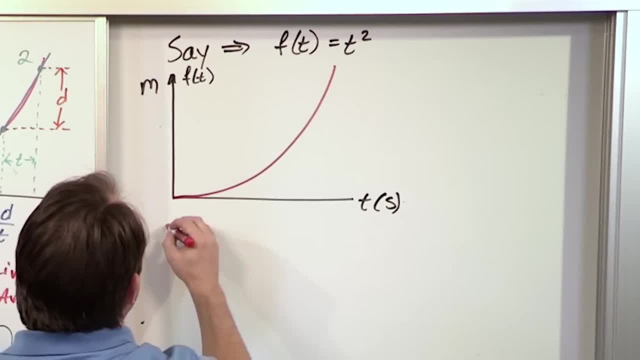 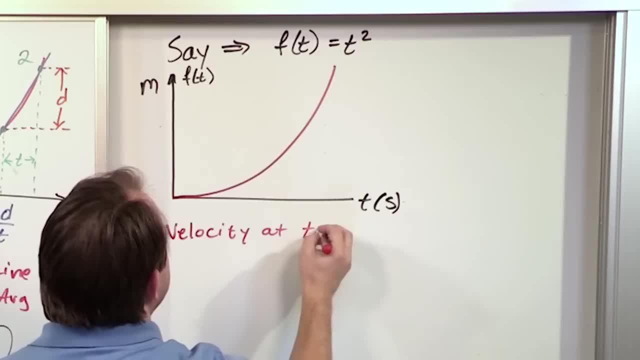 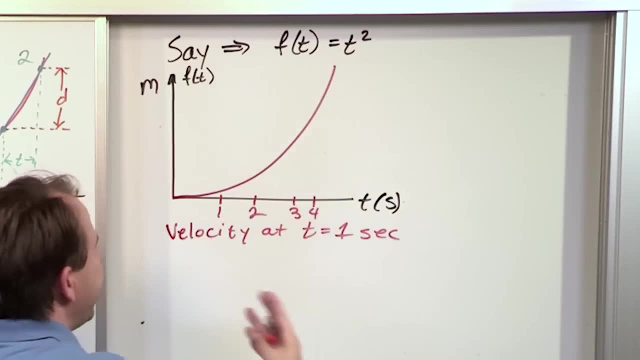 the velocity. What is velocity? What is the velocity? What is the velocity At? t is equal to one second. So here's some tick marks: One, two, three, four. one, two, three, four. So what this problem is asking is, even though the rock is constantly accelerating, the whole. 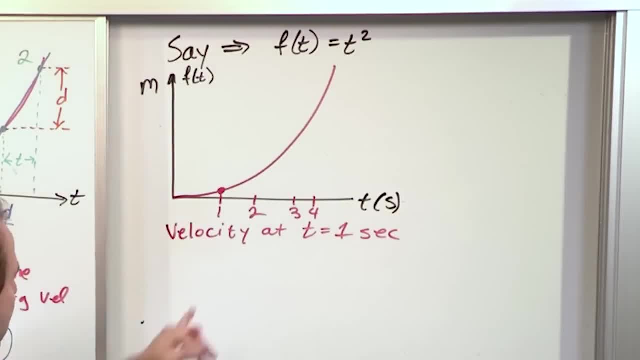 time. what is the velocity at this point right there on the graph? We don't want to know what it is here. We don't want to know what it is here. We don't want to draw a line and get an average. We want to know what the velocity is right there at that point. 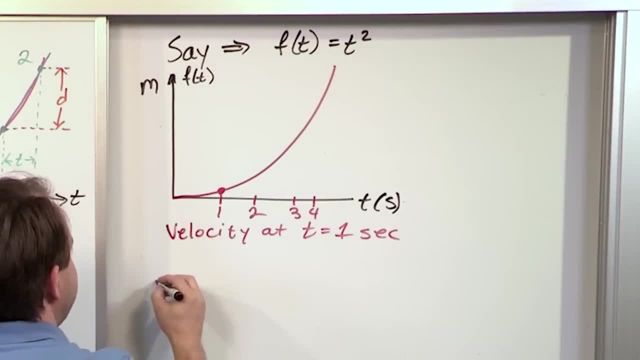 So we're going to use a limit to solve that. The equation we just write down has cold air blocked, tr술or, and so that's going to Survey about that�' & we'll pick reרג, which land here in a second, at a second in. 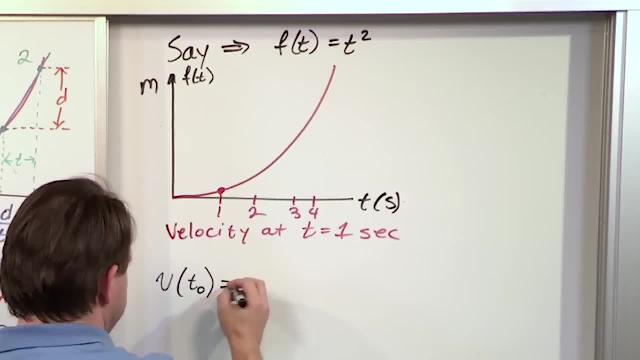 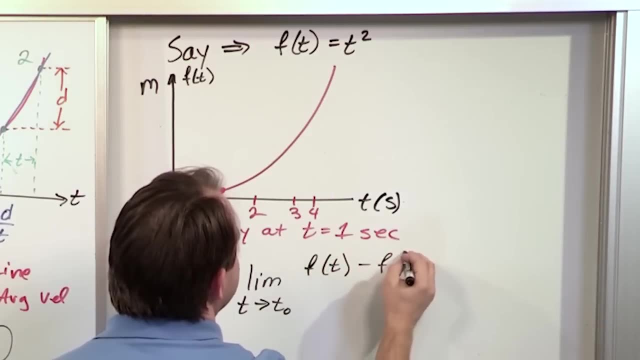 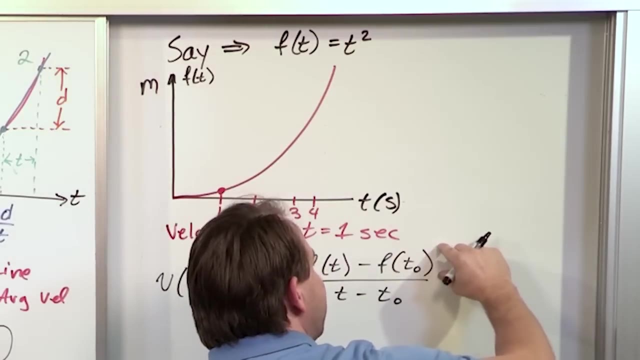 is the velocity, at whatever time t naught. we care about is the limit, as t goes to t naught of f, of t minus f, of t naught over t minus t naught. Don't forget what this equation is telling you. This is just the distance the rocket travels. 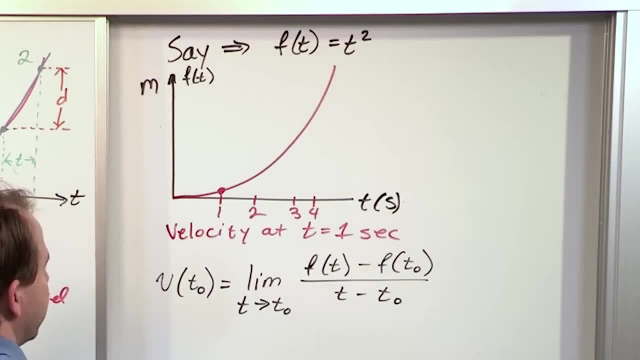 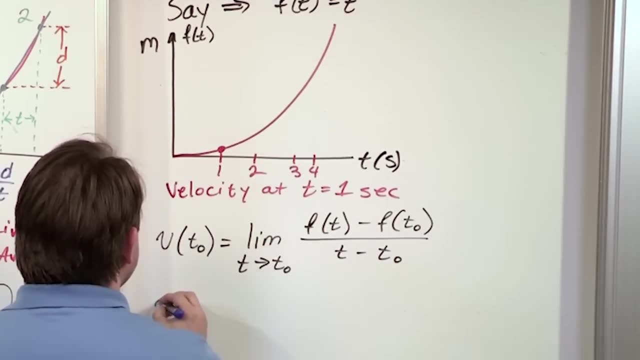 divided by the time the rocket does it, and we're sliding closer and closer. Now, in our particular case we only care about the velocity at t is equal to 1.. So we're going to rewrite this whole thing. So we'll say the velocity at t naught is 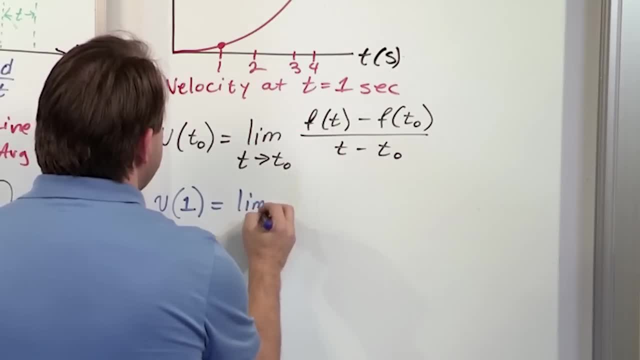 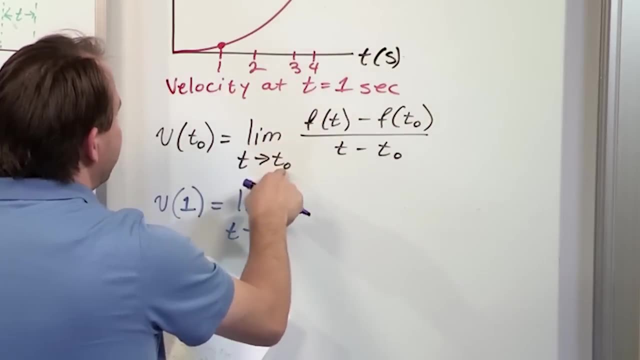 equal to 1 is equal to the limit, as t goes to 1.. Basically, everywhere this equation is written in terms of whatever time you want to find the velocity. So here is 1 second. We just replace 1 second everywhere that we see a t naught. 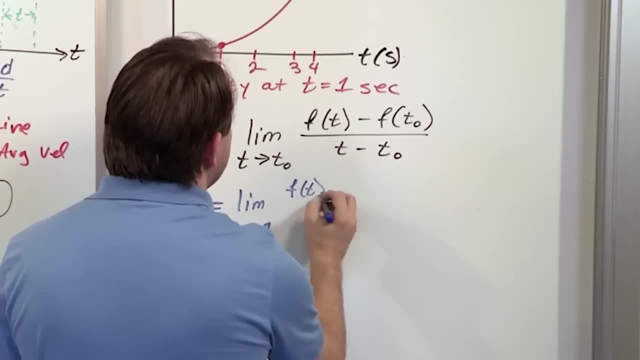 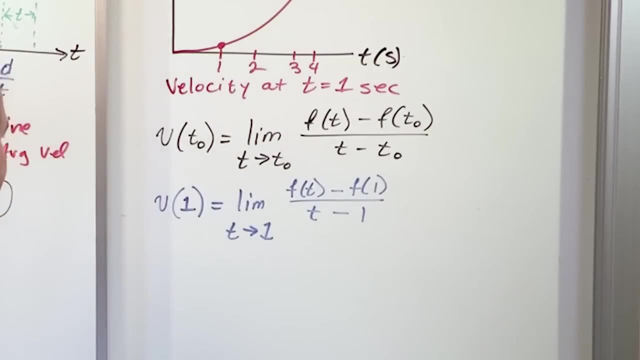 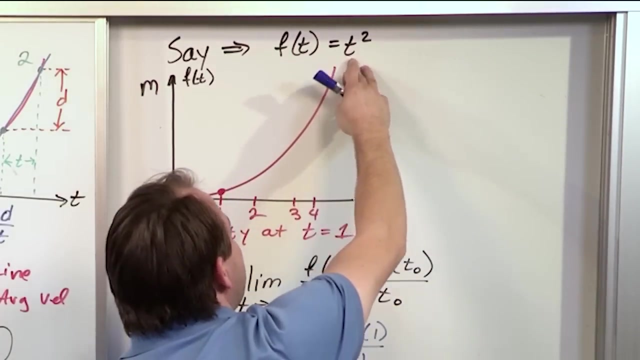 And then over here it'll be f of t minus f of t naught, so f of 1 over t minus 1.. But we know right, we know that the function of time for this particular rocket is actually t squared. So every second in time, the distance traveled up, we just square the. 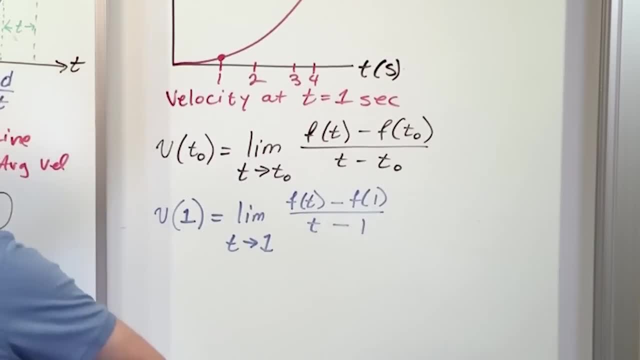 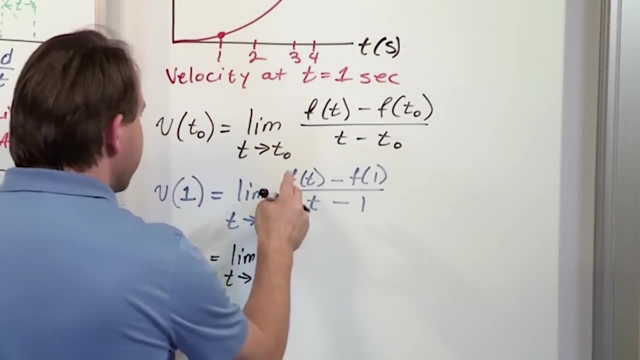 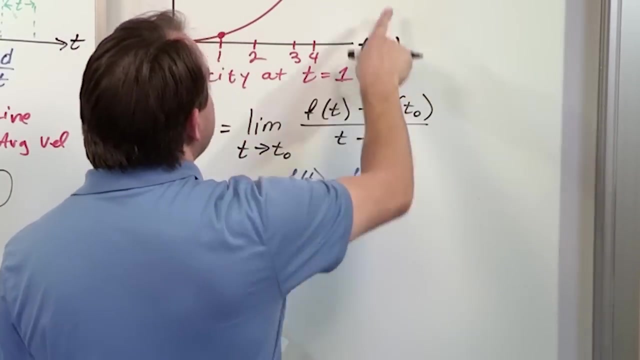 time, and that's basically the position on the graph. Okay, so now we know that this is equal to the limit, as t goes to 1 of what is f of t. We're given in the problem that that's t squared minus what is f of 1? If I take the value of 1 and I 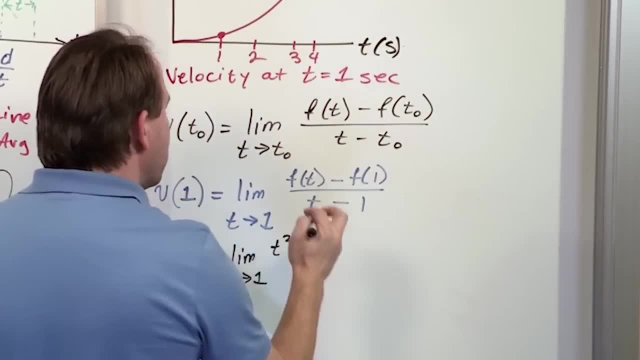 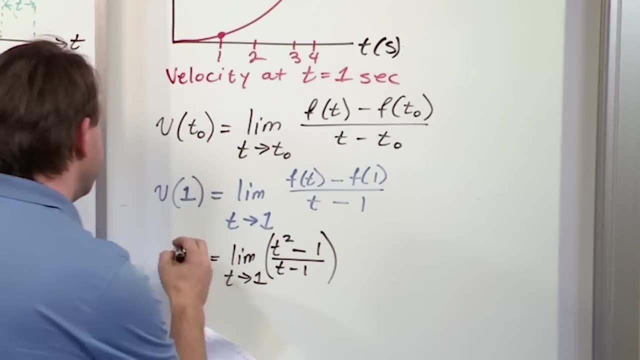 stick it into here: f of 1 is 1 squared, Which is just 1.. So this becomes a number And then on the bottom it's just t minus 1.. Now the entire problem: the velocity at 1 second is reduced to a limit problem, And 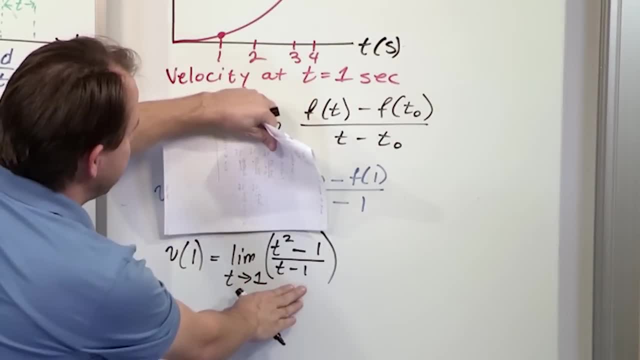 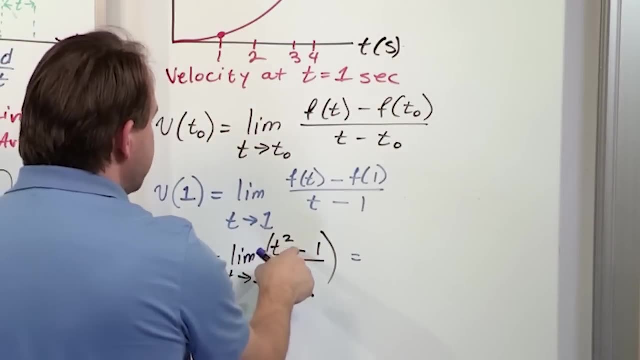 if I had covered all this stuff up and just told you to solve this problem. we've done a million of these. you know how to do that, So let's do it Over here. we first try to plug it in right, But we have 1 minus 1 on the top and 1 minus 1. 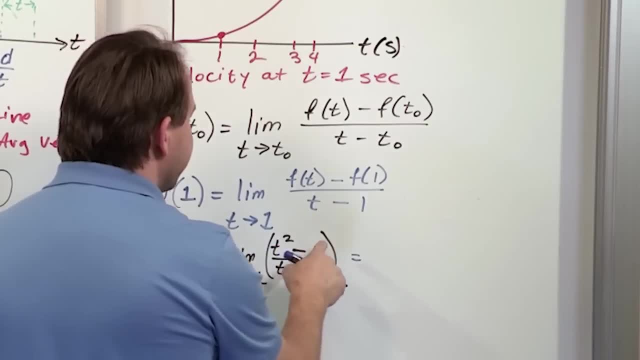 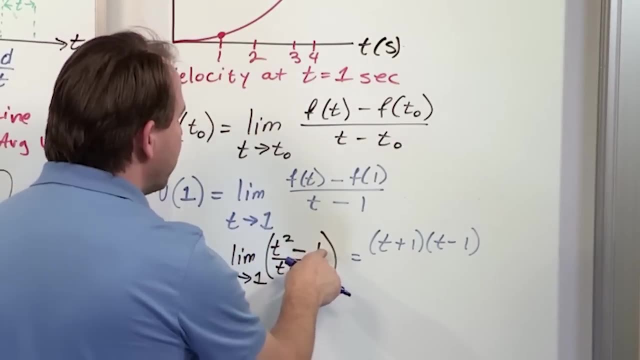 on the bottom, so we can't do that. But then we notice this is a difference of two squares on the top. So you write this as t plus 1, t minus 1, because this is t squared minus 1 squared, so it's a. 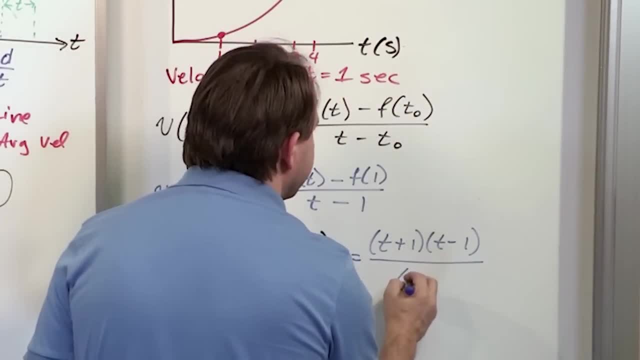 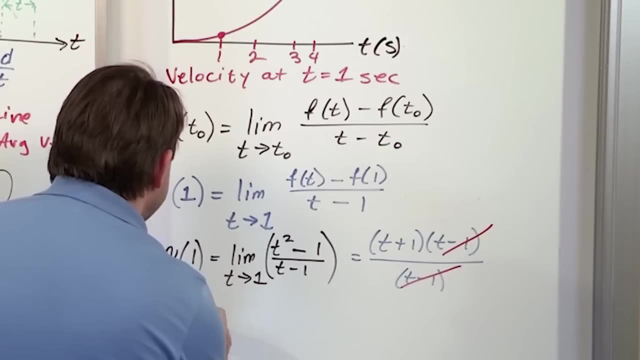 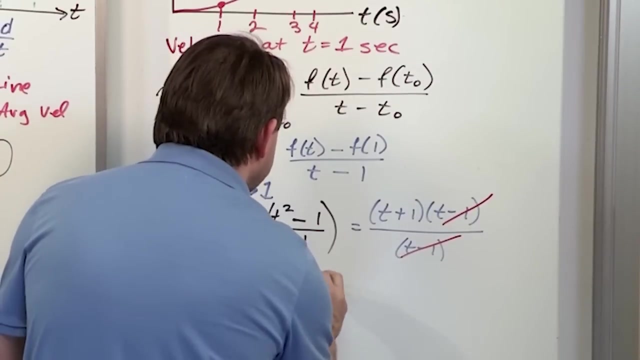 difference of two squares. On the bottom it's just t minus 1.. Now, of course, we do this only because it cancels. So the velocity at t is equal to 1 second is equal to the limit as t approaches 1 of what's left over, which is t plus 1.. Now 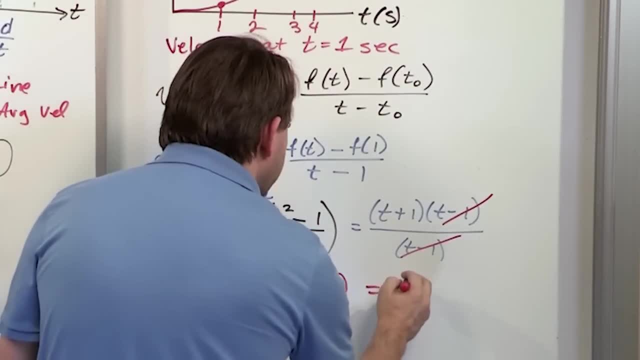 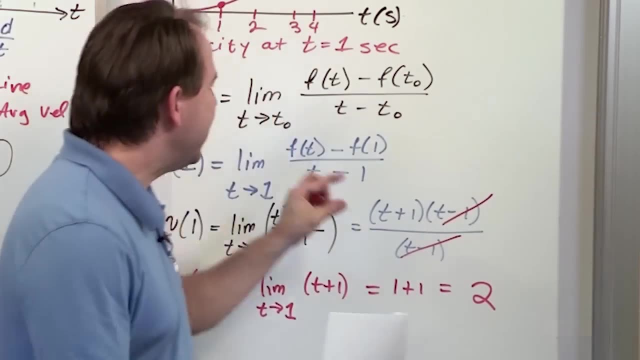 we try to plug in again, We can now see we can plug it in: 1 plus 1 is equal to 2.. Now, since we're dealing with distance and we're dealing with time and the original equation is calculating distance on top divided by time on the 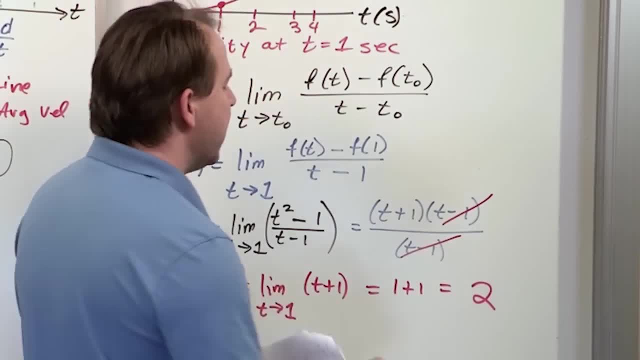 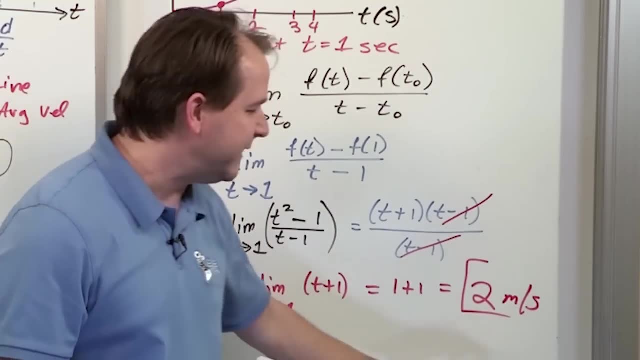 bottom it's meters, that's distance per second, which is time. So if we're dealing in meters and second, it'll be meters per second. If we were dealing with kilometers and hours, it would be kilometers per hour, but it is a velocity because of 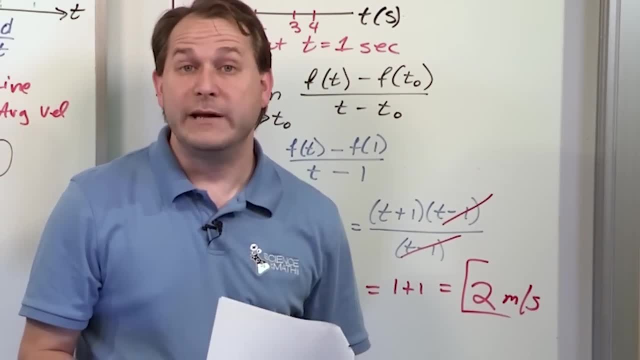 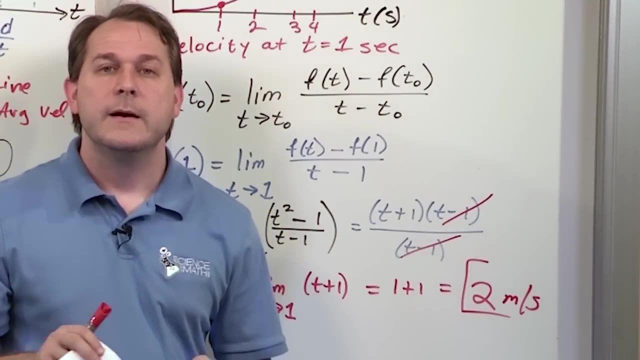 the units of our calculation. So what we've got is 2 meters a second. So, believe it or not, I know that was a lot. believe me, I do know it's a lot, but you have really just experienced one of the. 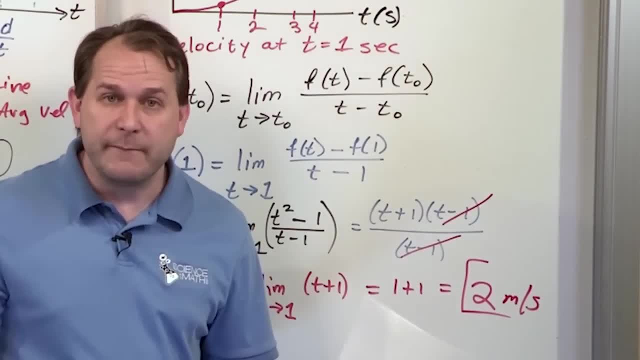 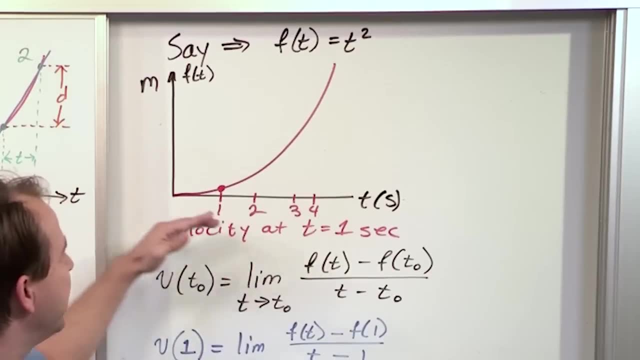 greatest intellectual breakthroughs in all of math. Because before calculus was invented, before this thing called a limit, before any of the stuff, it would have been impossible for us to even build a rocket, because we wouldn't know how to calculate how fast the thing was going when everything changes, I mean you. 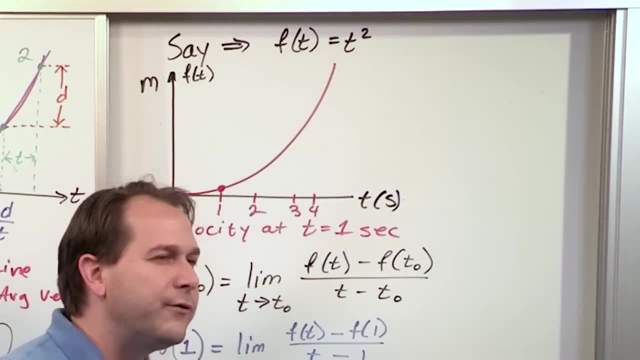 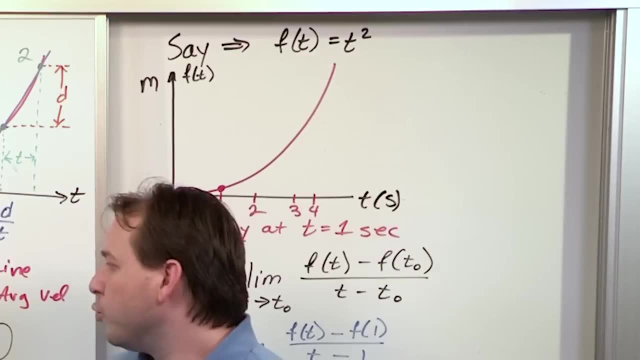 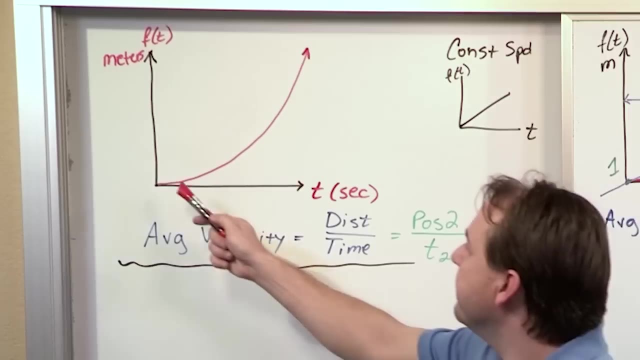 can look at two points and you can get a good idea, but you could never actually theoretically reduce the thing down to one point without the concept of a limit. Okay, so real quick recap: The main, main, main thing here is that when the 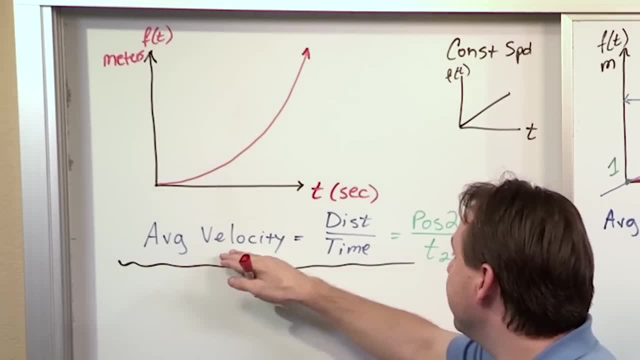 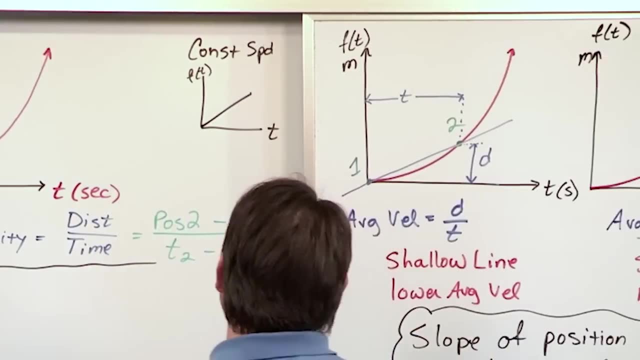 position of something is changing all the time. we can define an average velocity where we look at the two positions and divided by the two times distance over time, but it's just an aggregate average. It's not really great because it's averaged over two different positions. So we see the velocity here is. 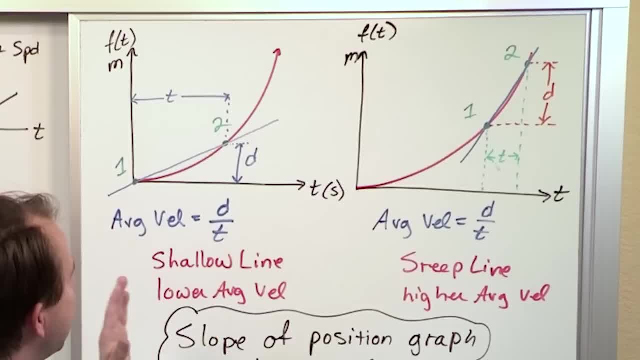 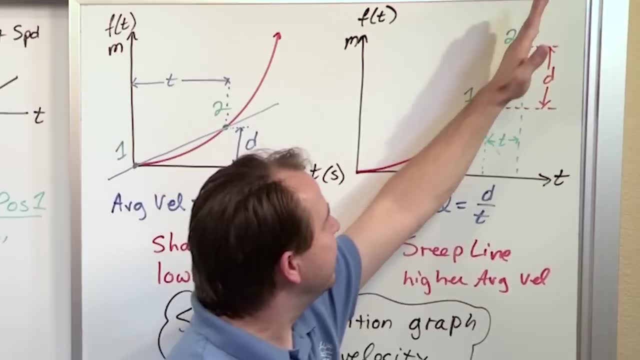 lower than the velocity. here. It gives us a good rough outline of it, but it's not exactly what we want. We see, this is a shallow line corresponding to a lower velocity, and this is a steeper line corresponding to a higher velocity. 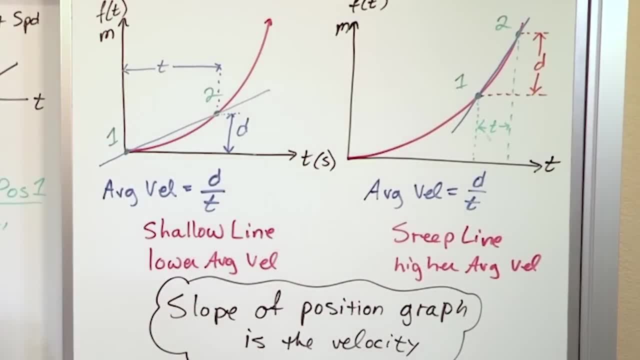 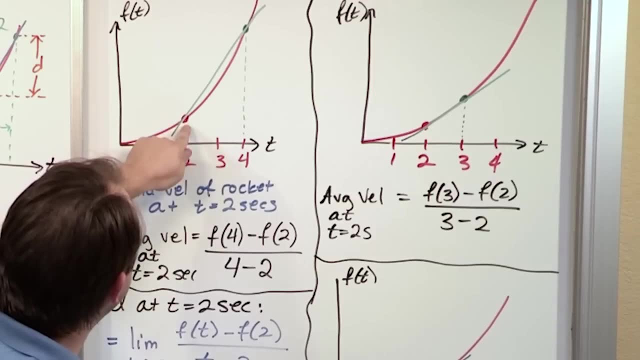 The slope of the line that you get when you do this basically corresponds to the velocity. So we do the whole thing again with numbers and then we say, well, if we want to know what the velocity is here, we can choose a point far away and we'll. 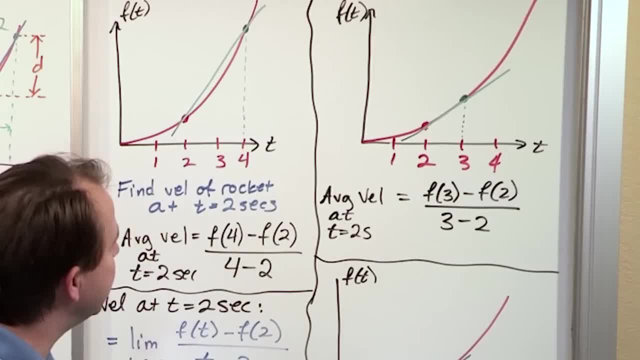 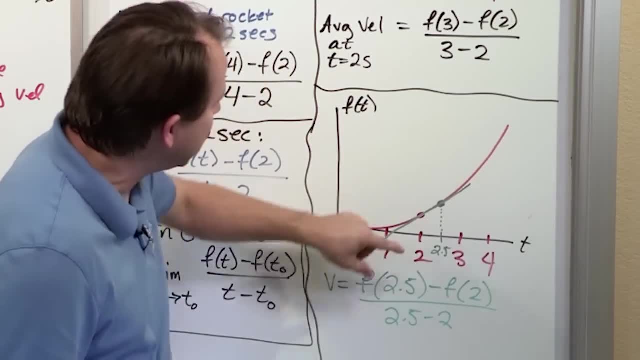 calculate the distance that we've risen divided by the time it took to do it, and then we'll move that point closer. and calculate the distance the rocket went up, divided by the time it took to do it, And then we'll move the point even closer and find out how far the 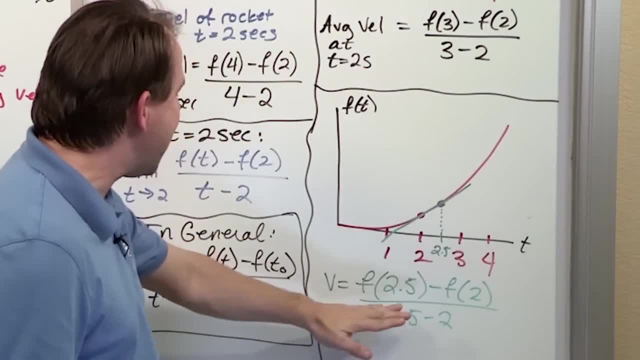 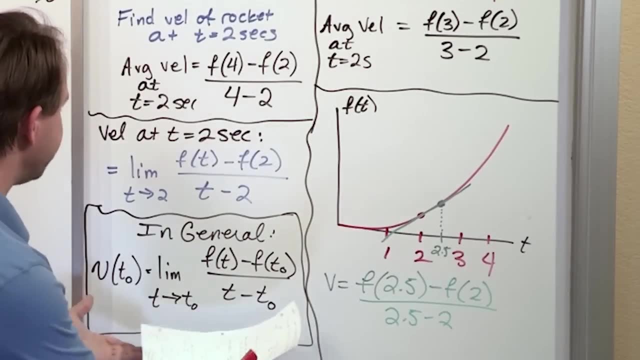 rocket moved up, divided by how far or how long it took for that to happen, We'll get a more accurate value of the velocity every time we do that. If you take it to its logical conclusion, then you get a general formula like this, where I can find the velocity at any point on this graph by just taking the. 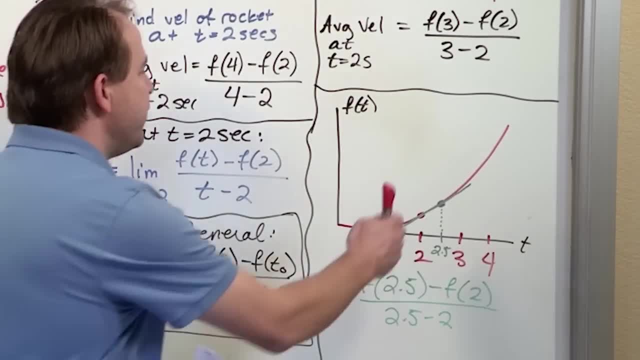 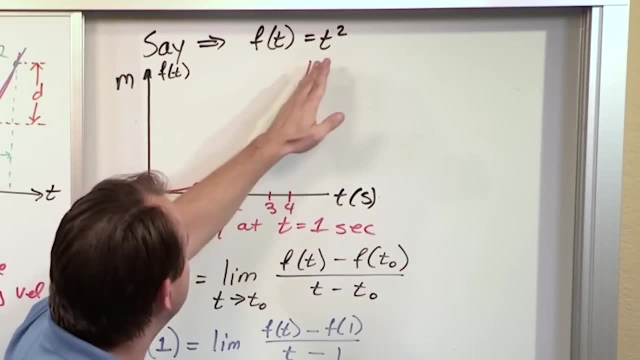 limit, as this value of t approaches the value of interest, just like we've done and divided by the difference on the bottom there. So we applied that to a real problem where the actual function was given, and then we get the value of t.